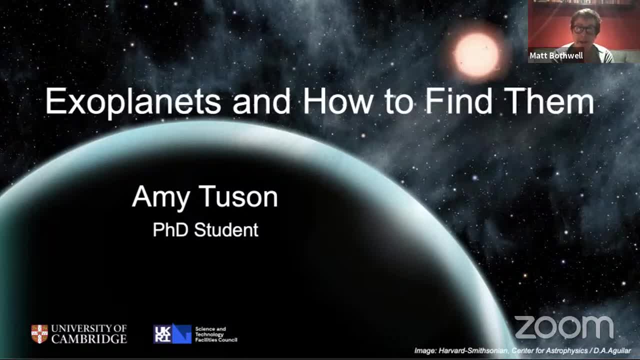 I'm very excited about this one. I'm here with Amy Toussaint. she's a third year PhD student in the Cavendish Astrophysics Department, where she studies exoplanets with Professor Didier Quelloz, and today she's going to be telling us all about exoplanets and how we find them. 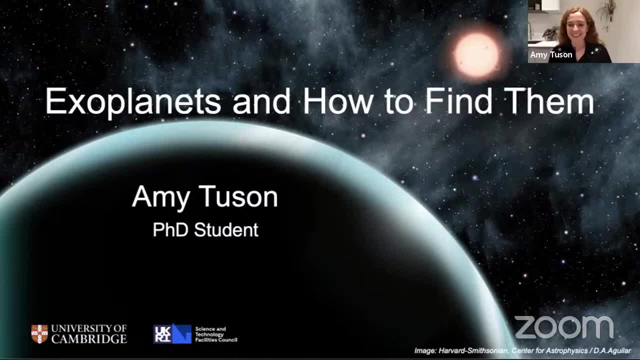 So over to you, Amy. Thank you, Matt. Good evening everyone. So, as Matt said, my name is Amy Toussaint and I'm a third year PhD student working with Didier Quelloz here at the University of Cambridge. 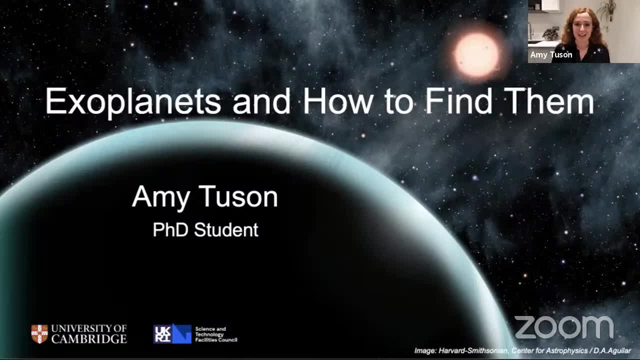 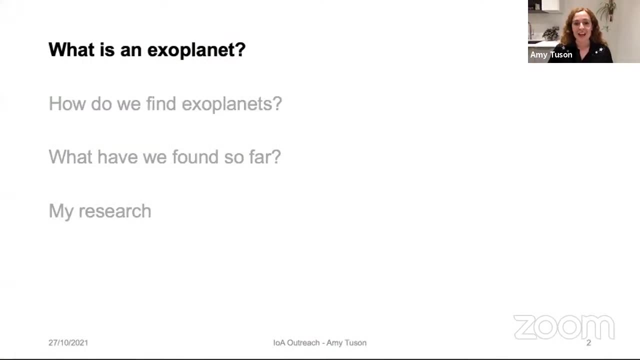 Tonight I'm going to give you an introduction to exoplanets and the research I'm doing, And then I'm going to show you how you can get involved in the search for exoplanets at home. So to start with, what is an exoplanet? It's defined as any planet beyond our own solar system. 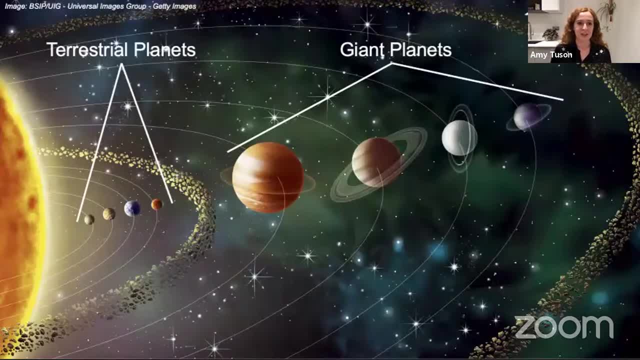 Let's think about what that means by first looking at our solar system. So there are eight planets in total: The interterrestrial planets Mercury, Venus, Earth and Mars, which are all rocky like the Earth, and the outer giant Mercury, Venus, Earth and Mars, which are all rocky like the Earth, and the outer giant Mercury, Venus, Earth and Mars, which are all rocky like the Earth. 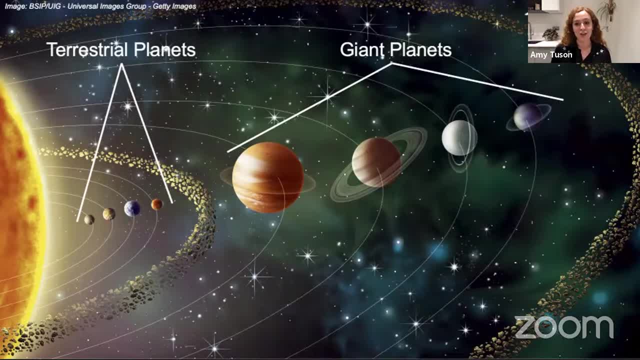 and also there are other giant planets. So Jupiter and Saturn are gas giants, whilst Uranus and Neptune are ice giants. Because they're so far away from the Sun they're very cold. All eight of these planets are orbiting our host star, the Sun. 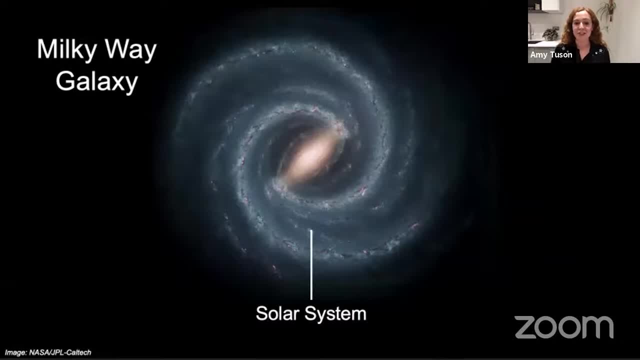 But there are many more stars. The solar system is about here, in one spiral arm of our host galaxy, the Milky Way. They're estimated to be about 250 billion stars in our galaxy and there could be planets around almost any one of them. These are the exoplanets. 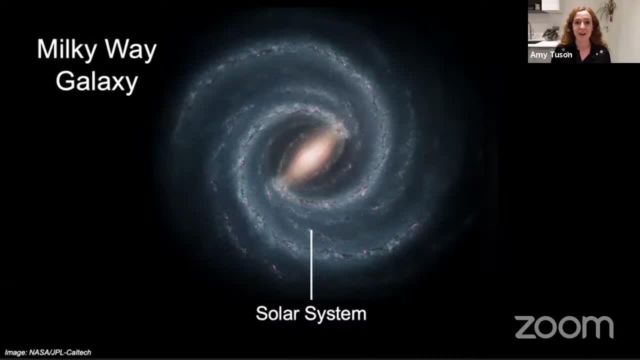 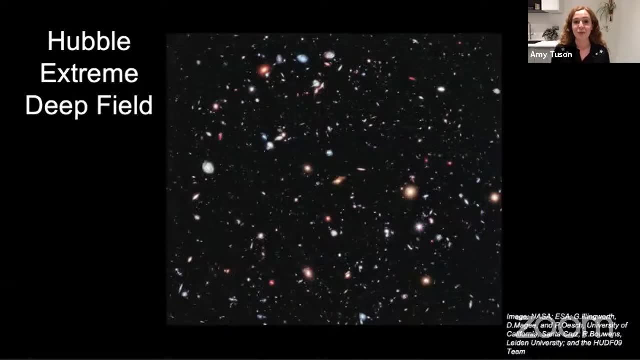 we're talking about a planet that orbits any star other than our sun. And the Milky Way is not the only galaxy. There is a whole universe of galaxies. This image shows the Hubble Extreme Deep Field. It's a patch of sky smaller than the full moon, yet it reveals over 5,000 galaxies. 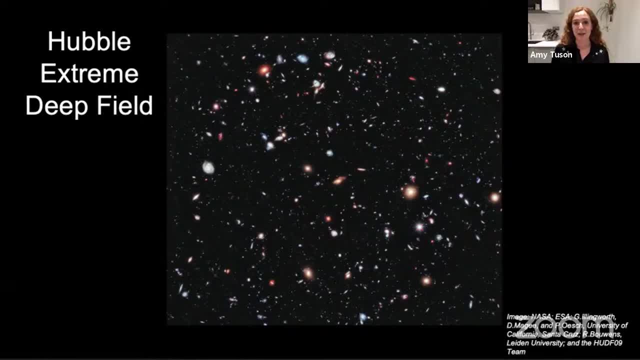 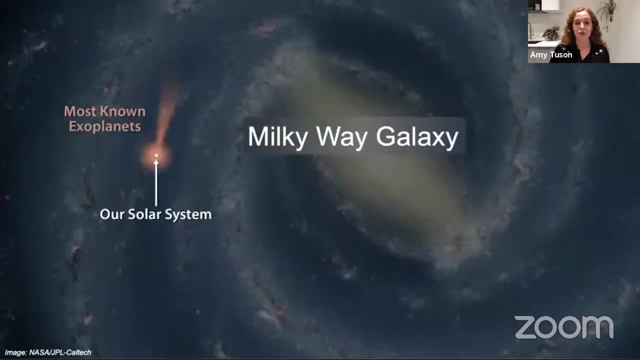 Each galaxy contains billions of stars and just as many planets. However, all of the exoplanets we've found so far are within our own galaxy. Not only that, but we've only really observed a very small fraction of it, So that's shown here where. 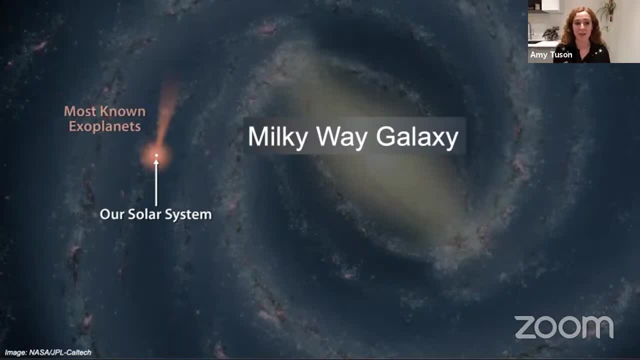 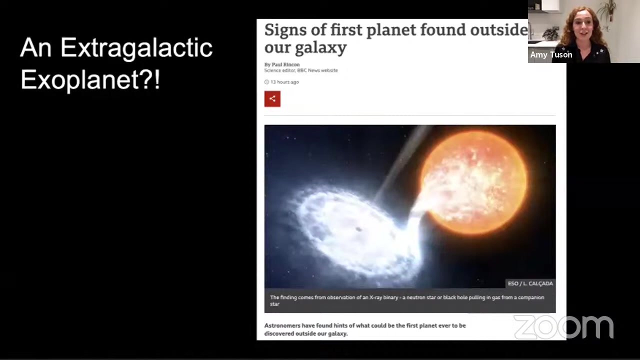 we can see, most known exoplanets are in a bubble around our solar system, And that's just because observing exoplanets around distant stars is much, much more difficult. That makes this week's exoplanet news even more amazing. Astronomers think that they've found: 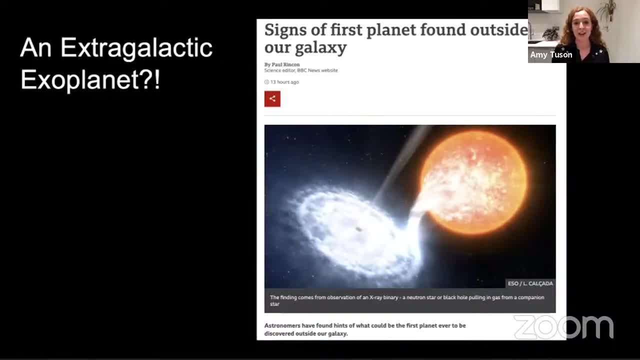 signs of the first exoplanet outside of our galaxy. They need more data to confirm if it really is an extragalactic exoplanet, But the study opens up a whole new way to find exoplanets at much greater distances than ever before. So we know the planets are out there, but how do we find? 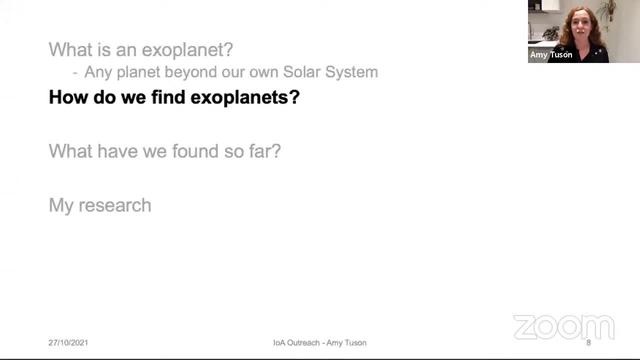 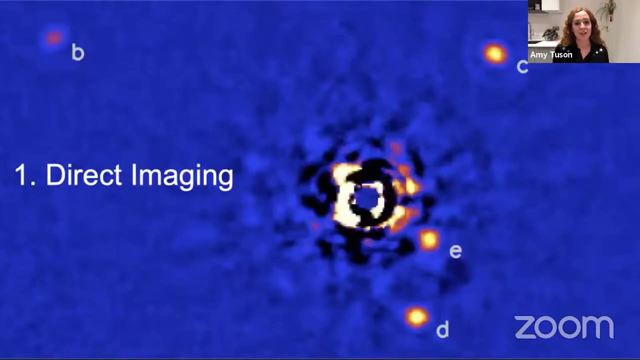 them. So far we have over 4,500 confirmed exoplanets, and astronomers have a few techniques to help find them. The first idea you might have is to try and take a picture of an exoplanet. So this is a really nice example of four planets labelled b, c, d and e orbiting a star. The only reason we're able to see these planets is because they orbit far away from their star. they're big and they're young. Only about 50 exoplanets have been found using imaging, because it's not very often that we get this perfect combination of properties. Consider taking a picture of a plane near the sun. The bright light from the sun would obscure the image and you wouldn't be able to see the plane at all. We have exactly the same problem when we try to image exoplanets orbiting distant stars. 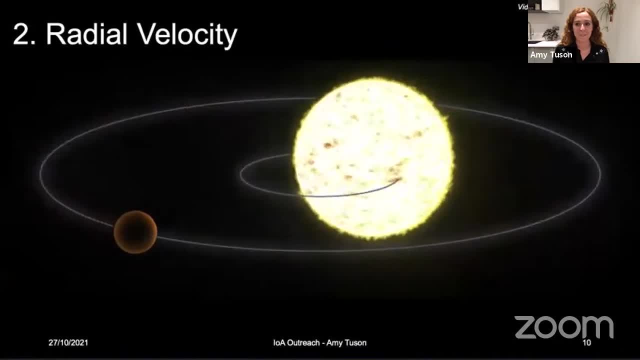 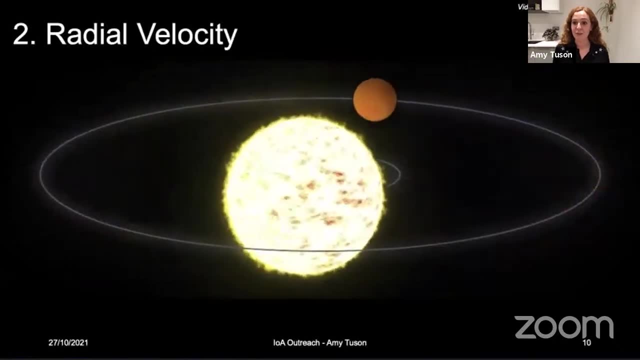 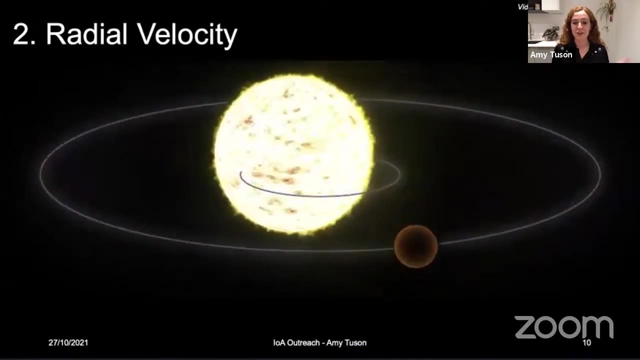 An alternative method is radial velocity, So the force of gravity acts between any two objects in the universe. It acts between you and the earth, which keeps you firmly planted on the ground. It also acts between a star and a planet, So the star is a lot more massive and therefore exerts. 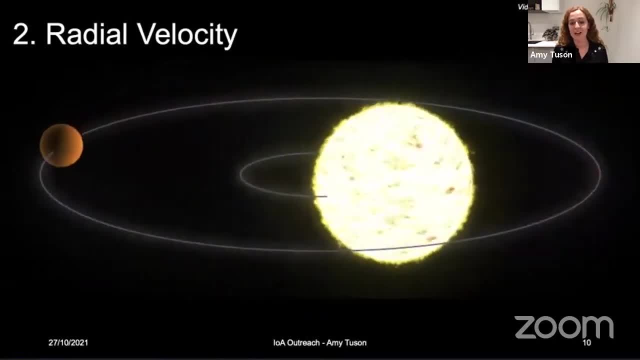 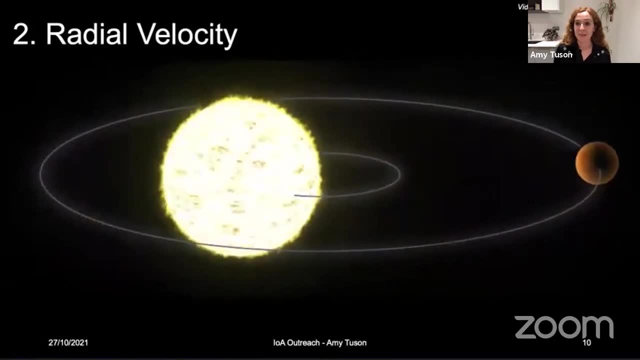 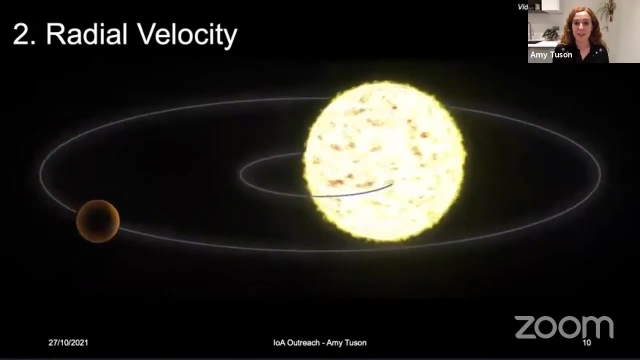 a strong gravitational force on the planet, And so we typically think of the planet as orbiting the star. But even though the planet is much smaller, it still exerts a gravitational pull on the star. So look at this animation. You see how the star is moving- a little bit too. 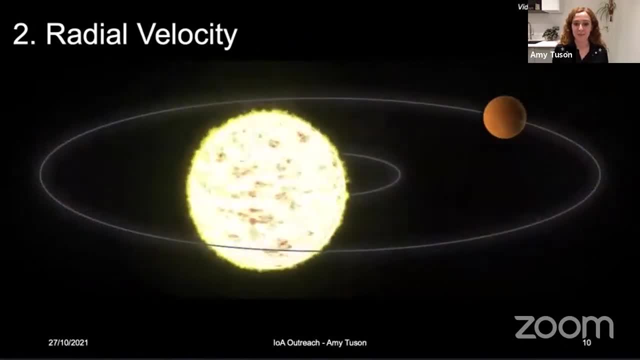 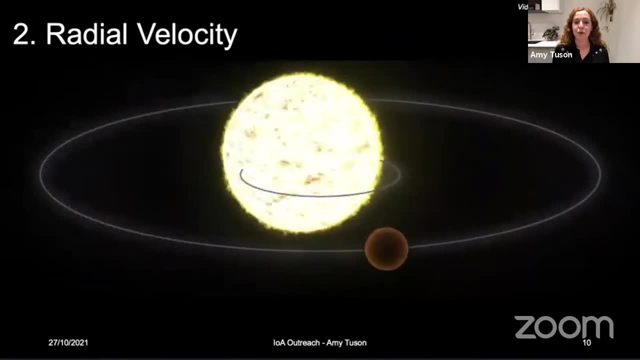 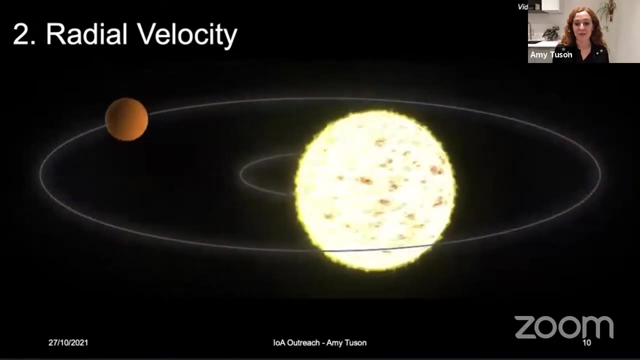 The planet's gravity is causing it to wobble in this way. The more massive the planet is, the bigger the effect it has on the star. So measuring a star's wobble can therefore tell us if a star has planets orbiting it, and it can provide an estimate of the 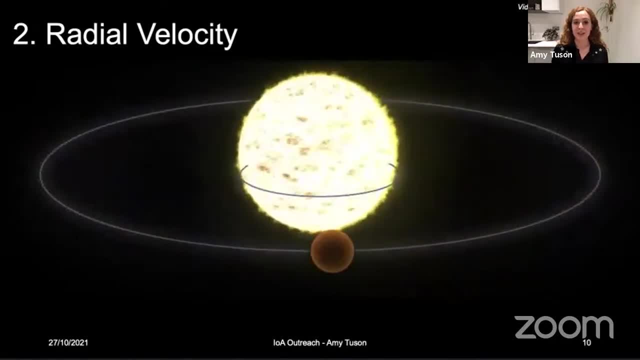 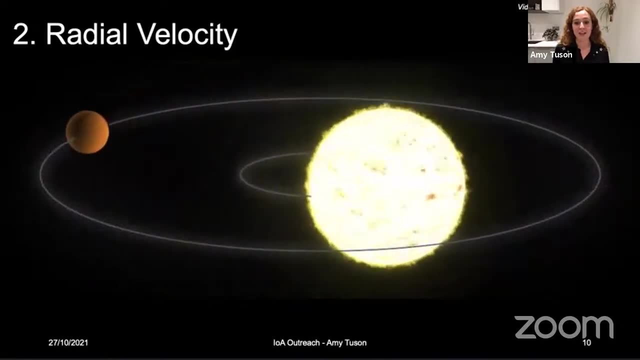 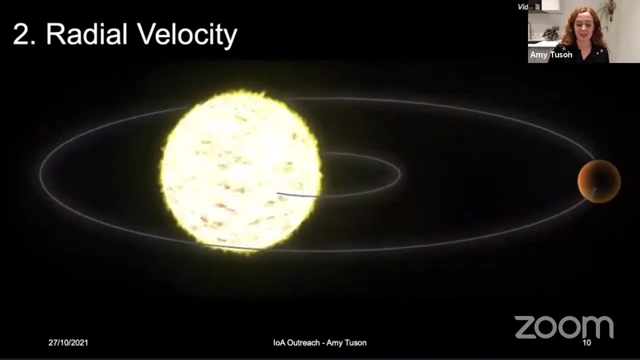 planet's mass. Didier Coelho's and Michel Maillot's discovery of the first exoplanet around a sun-like star in 1995 was made using the radial velocity method, And since then this method has discovered nearly 900 exoplanets. For the final discovery method I will discuss first, consider: 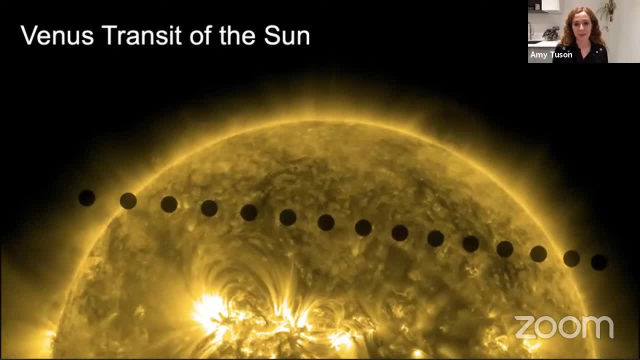 have you ever seen a planet transit across the sun? It happens when one of our intelligent, curious solar system planets, either Mercury or Venus, passes between the Earth and the Sun, So this image shows the 2012 transit of Venus. A series of images were taken from space by NASA's. 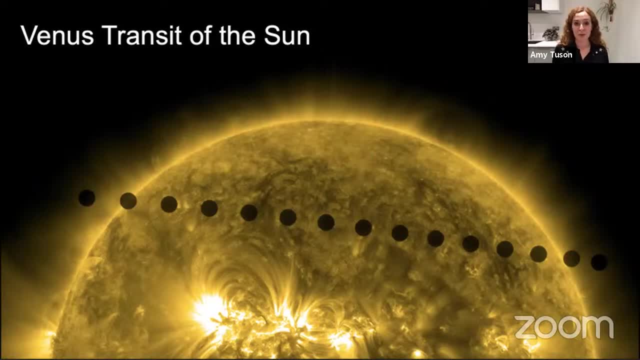 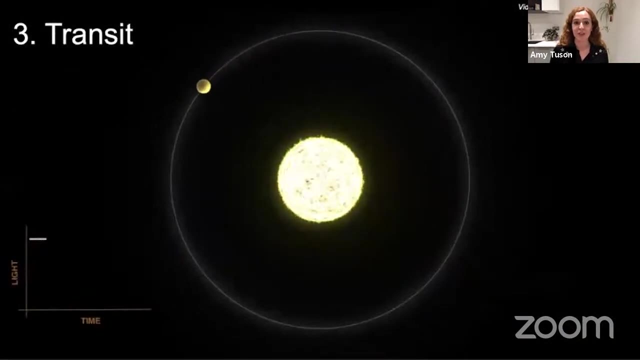 Solar Dynamics Observatory and then combined to produce this final, really cool image of the entire transit event. So you can see the path that Venus traced as it went in front of the solar disk. The transit method is based upon the same concept as shown in this animation here, So it's the most. 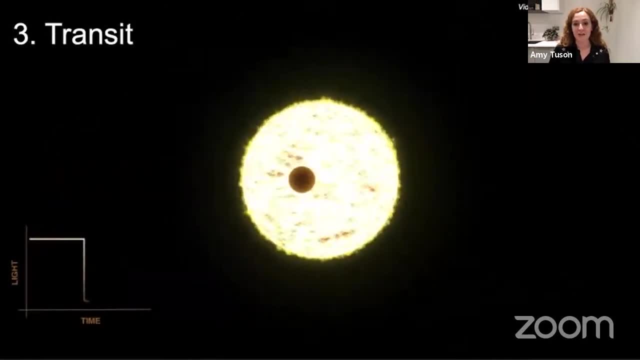 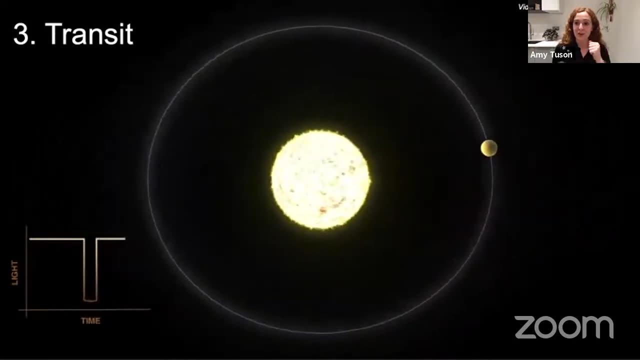 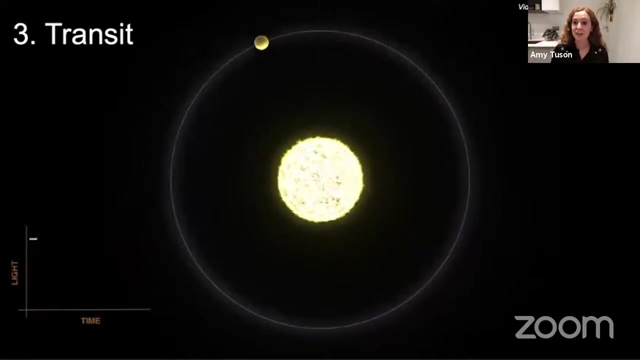 successful method to date, boasting the discovery of almost 3,500 exoplanets. If you imagine that you're the observer when the planet passes between you and the star it orbits, it blocks some of that star's light, So a telescope pointed at the star will detect a small decrease in the amount of light. 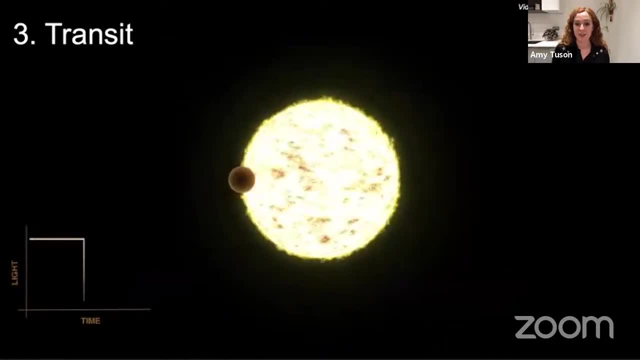 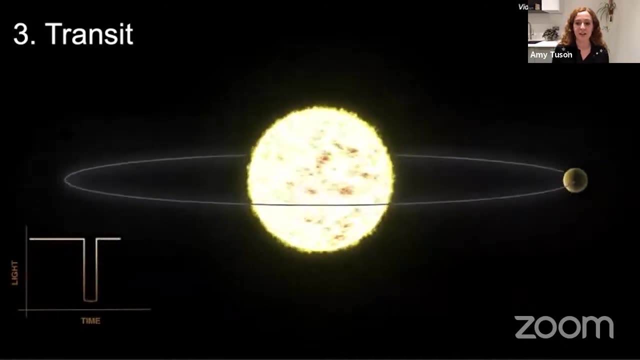 This indicates the presence of an exoplanet around a distant star. The graph being plotted in the bottom left is called a light curve. It shows the amount of light arriving at the telescope over time, And that light curve clearly shows a drop in brightness. 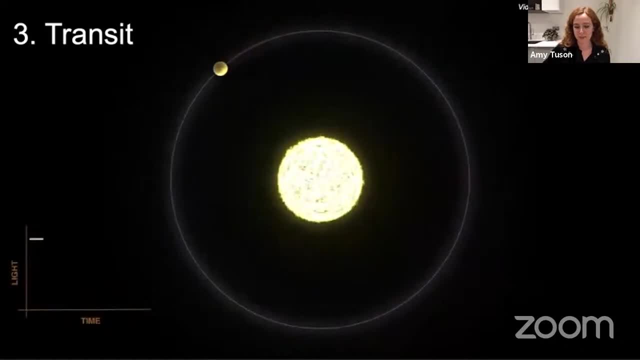 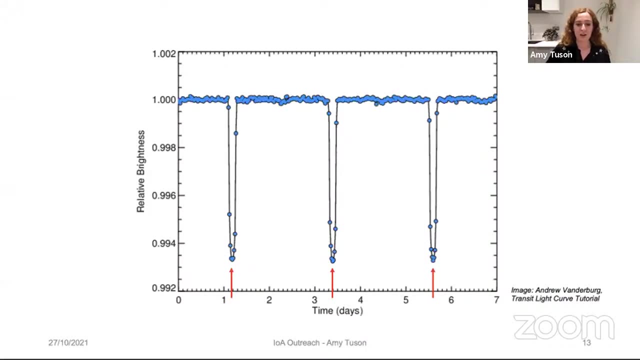 caused by the planet passing in front of the star. So let's look more closely at an example light curve. There are three big drops in brightness highlighted with red arrows, And these correspond to transits of a planet. Typically, you need at least three transits to 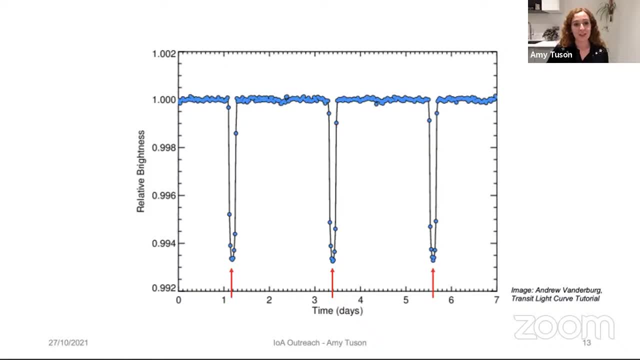 be able to confirm an exoplanet. So, using this light curve, we can gain some valuable information about the system. The separation between two transits corresponds to the orbital period of the planet. This is the time taken for the planet to complete one full orbit of its star. So, in the case of the earth, 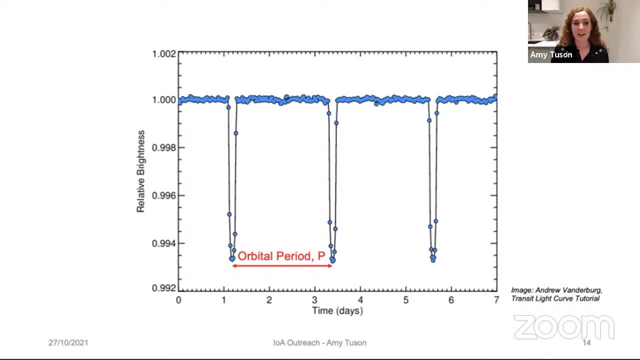 this would be 365 days. In other words, the orbital period tells us how long one year would be on these planets. Furthermore, the depth of the transit can be used to calculate the radius of the planet. A big planet will cause a deeper transit than a small planet, because it blocks. more light from the star. These three transits are caused by a big, Jupiter-sized planet, so they're very deep and easy to see. If we instead had a smaller, Earth-sized planet, the transits would be much, much shallower. For example, there is an Earth-sized planet. 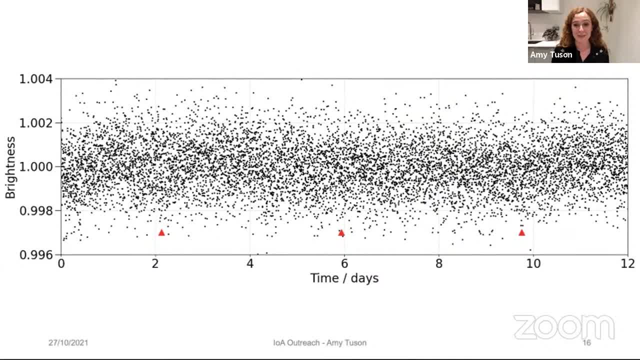 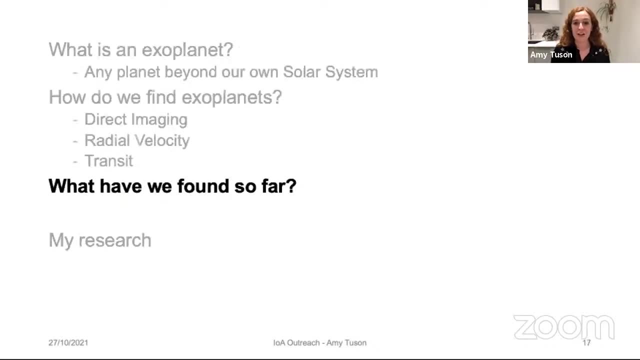 hidden in this data. You probably can't see them, neither can I, but the positions of the transits are indicated by the red triangles. Due to the very shallow transits, small planets are therefore much more difficult to find. So we've understood what an exoplanet is and how we can find them. We now want to explore. 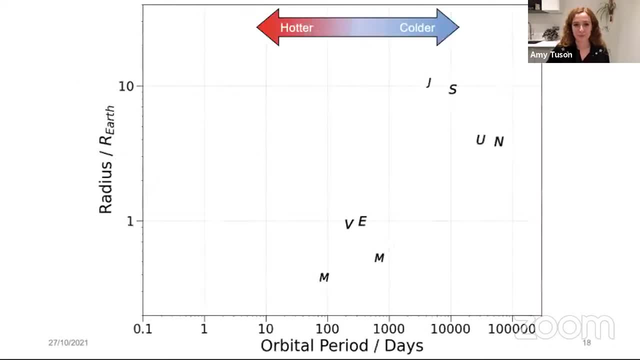 the exoplanets we've discovered so far. Let's start by looking at this plot of orbital period against radius, showing just the solar system planets, So the axes. here we have orbital period in days along the bottom and we have radius compared to the Earth, For example. Jupiter has an orbital period of about four and a half thousand days and a radius of about ten times the Earth's radius. So remember that a shorter orbital period means the planet is closer to the star and hence it's hotter than a planet with a long orbital period. 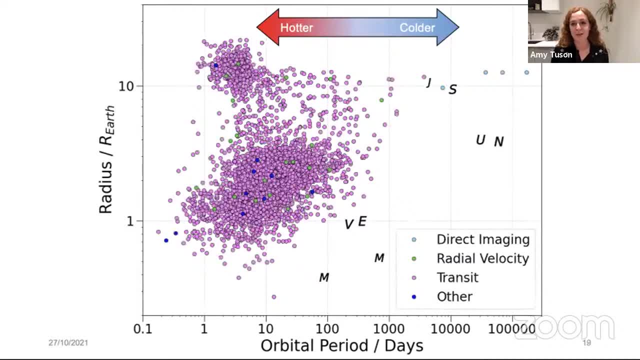 So we can now populate this diagram with all of the confirmed exoplanets that have both a period and a radius measurement, And these points are coloured according to what method was used to discover the planet. So pale blue is direct imaging, green is the radial. 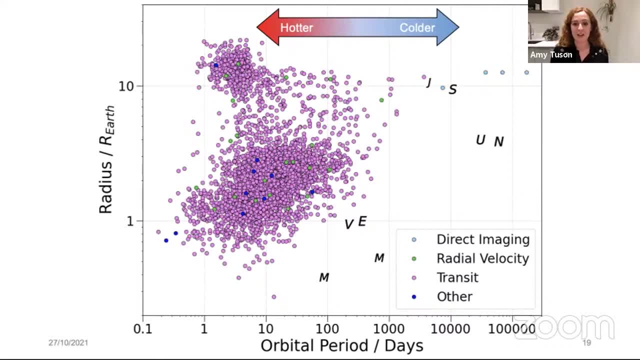 velocity method and pink is the transit method. There is an incredible variety of exoplanets covering a really large range in size and orbital period, So we can begin to make sense of them by classifying the planets based on their radius. Firstly, the planets with the largest radius are the gas giants. These planets don't have solid surfaces. Instead, they have a solid core surrounded by vast clouds of helium and hydrogen. Notice that there's a big clump of gas giants, and these have a much shorter orbital period than Jupiter or Saturn, So this means that they're much hotter. 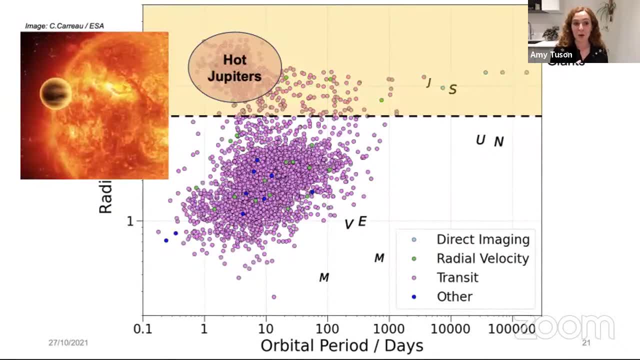 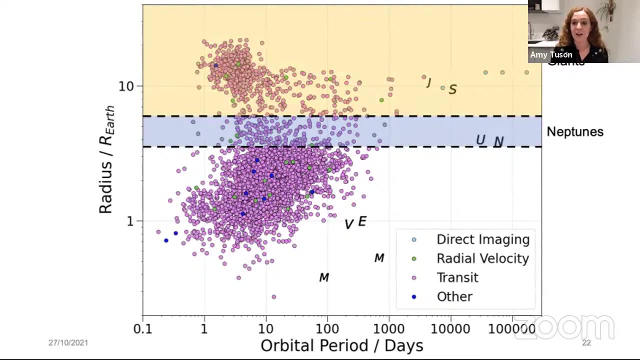 So, therefore, this cluster of exoplanets are referred to as hot Jupiters. They're unlike anything we see in our own solar system, and there's a lot of questions about how they work. Next are the planets with a radius similar to Neptune, So these typically have hydrogen. 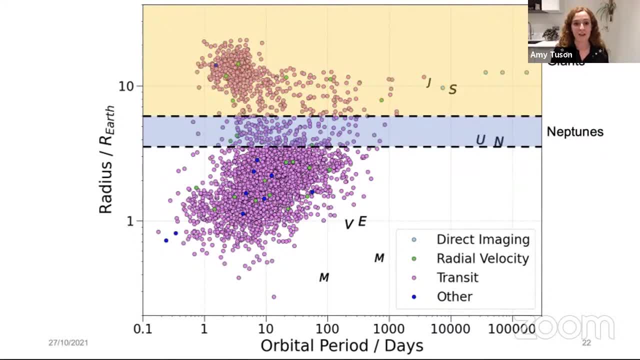 and helium-dominated atmospheres with cores of rock and heavy metals. Then we come to planets which are between the size of Earth and Neptune. These can be divided into two categories. So we have mini-Neptunes, which are scaled-down Neptune-like planets. 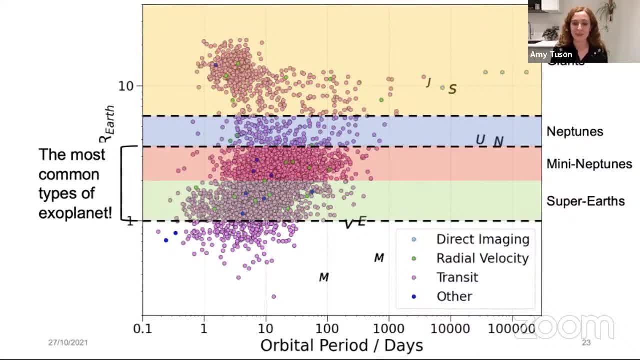 and super-Earths, which are scaled-up rocky planets. Mini-Neptunes and super-Earths are actually thought to be the most common type of planet out there, even though we see no such planet in our own solar system. Finally, we have the terrestrial planets. These are rocky planets that may or may not. have an atmosphere. We also have a special name for rocky planets orbiting very close to their host star. They are called lava worlds. So these planets are so hot that they're surfaced in the atmosphere. They're called lava worlds, So these planets are so hot that they're surfaced. in the atmosphere. So these planets are so hot that they're surfaced in the atmosphere. They're called lava worlds. So these planets are so hot that they're surfaced in the atmosphere. They're called lava worlds. So these planets are so hot that they're surfaced in the atmosphere. 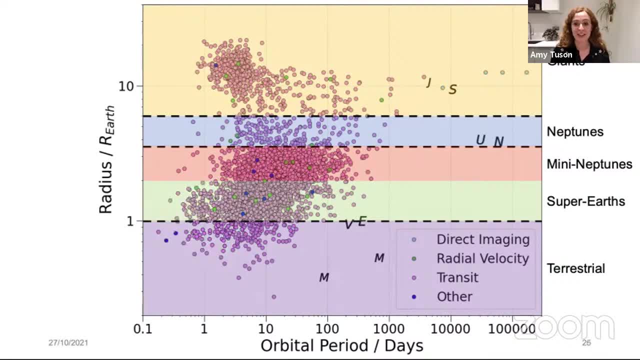 They're called lava worlds, So these planets are so hot that they're surfaced in the atmosphere. The key takeaway from this is that there is a vast diversity of planets out there. As discoveries continue to be made, we never fail to be surprised by what we find. The 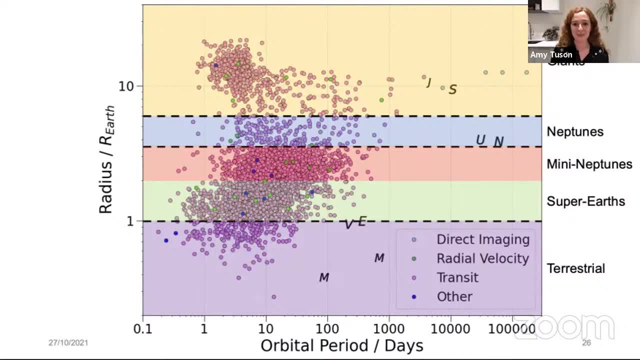 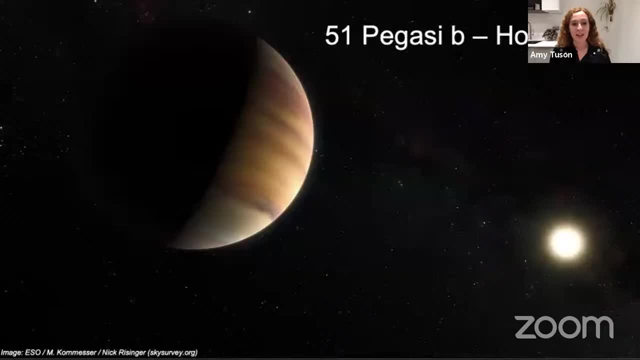 excitement of this field lies in not knowing what we might find next. So let's have a look at some of the exoplanets we've found so far. So here is an artist's impression of 51 Pegasi b, the first exoplanet that was discovered. 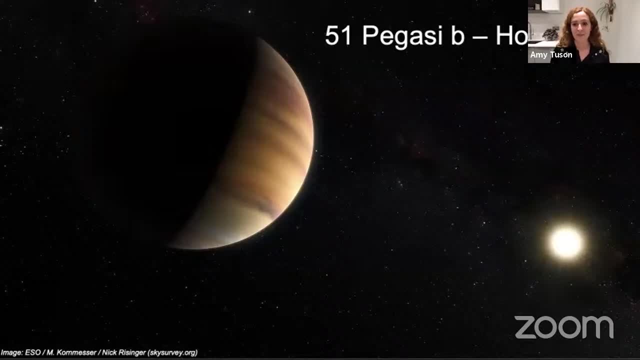 the first exoplanet ever discovered around a sun-like star, So it was actually discovered by my PhD supervisor back in 1995, when he was a PhD student himself. This planet was about half the mass of Jupiter, measured using the radial velocity method. and it orbits its host star every four days. So remember that means that it goes around the star once every four days, which is incredibly fast. The planet is therefore a hot Jupiter. However, it does not have a radius measurement, So, due to its proximity to the star, the atmosphere of this planet must be incredibly hot. 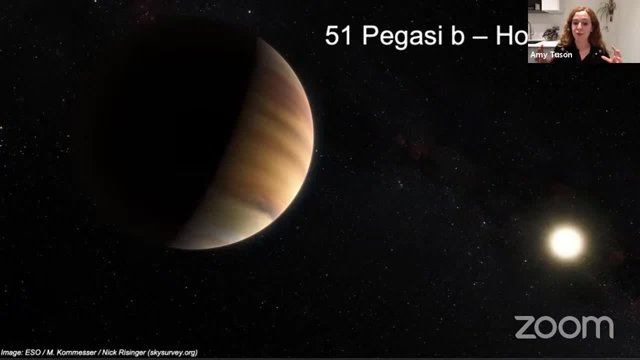 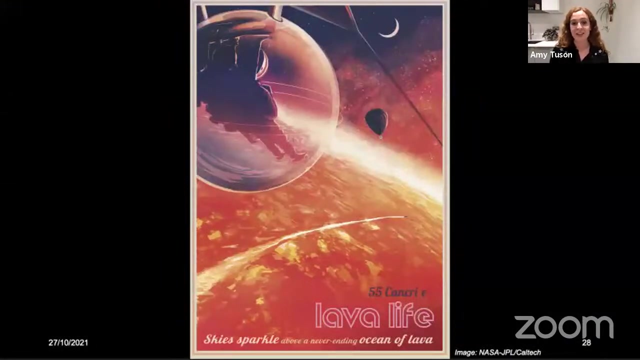 And astronomers think that this would cause the atmosphere to puff up, creating a really thick layer, meaning the radius of this planet is probably much larger than that of the Jupiter. in our own solar system, 55 Cancri e is a lava world, So it's a little larger than the Earth, making it a super-Earth planet, but it orbits its star in less than 18 hours. 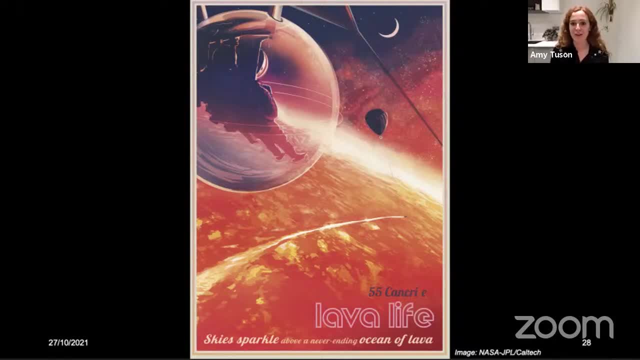 So one year on this planet is less than one day on Earth. This planet is so hot that the surface is lava that never cools enough for a crust to form, And, in fact, the surface is so incredibly hot that silicate rocks melt and the silicate vapour that would then be in the atmosphere might cause the cloud to collapse. 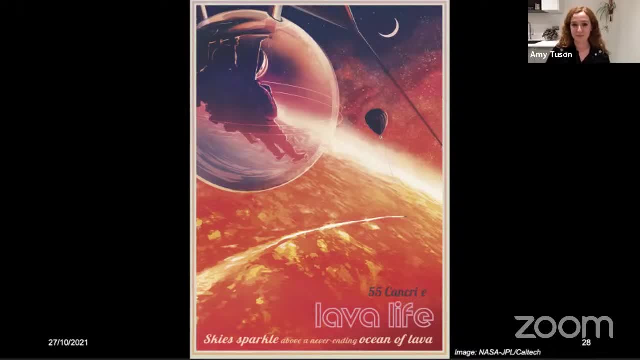 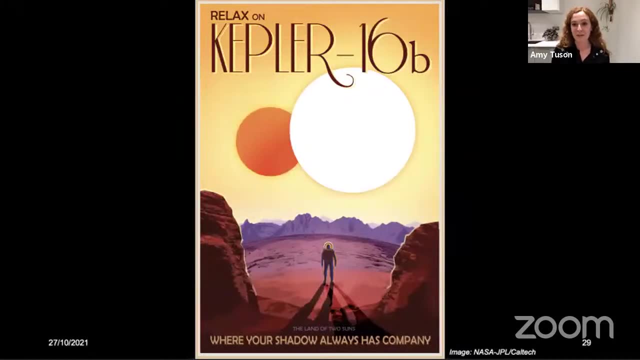 55. Cancri e is a lava world clouds on this planet to sparkle. Kepler-16b is a special planet that orbits a pair of stars, much like the famous planet Tatooine from Star Wars. So this poster depicts the surface of the 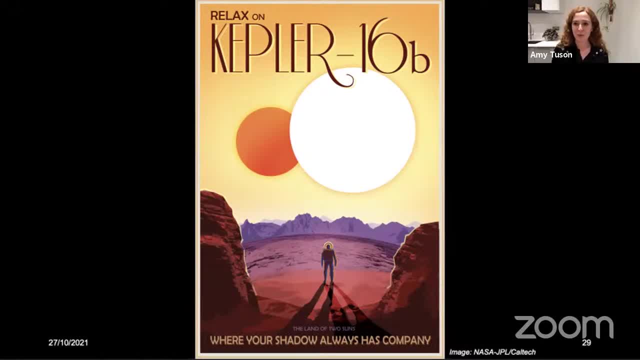 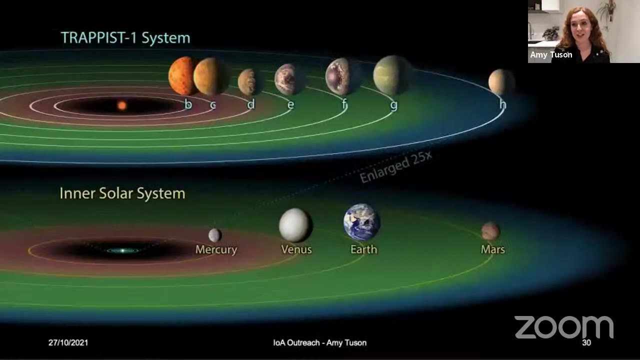 planet as rocky, but it could be a gas giant. we're not really sure. Although this planet wouldn't be suitable for life, its existence proves the iconic double sunset from the movie is far from science fiction. Finally, I'd like to show you an interesting exoplanet system called TRAPPIST-1.. 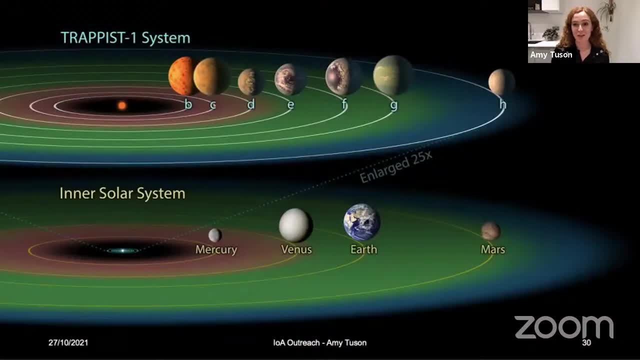 So this system contains a total of seven Earth-sized rocky planets orbiting incredibly close to their host star. If you look at this illustration, you can see that all seven of the TRAPPIST-1 planets lie well within the orbit of Mercury. in our own solar system, The green-shaded 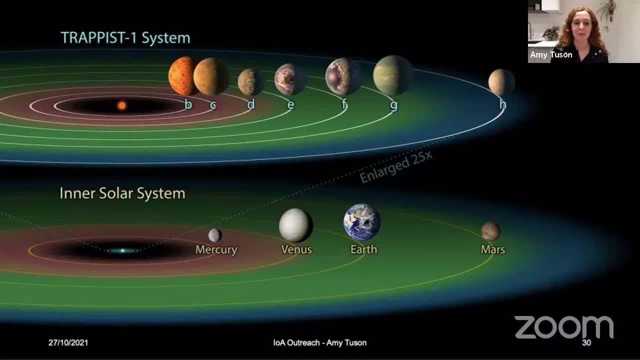 region represents a star and the star-shaped region represents a star. So this system is a special area which is called the habitable zone. So this is the zone where the temperature on the planet could be just right for liquid water to exist on the surface, a crucial condition for 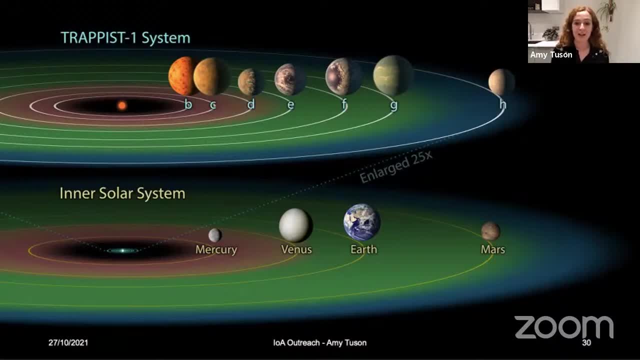 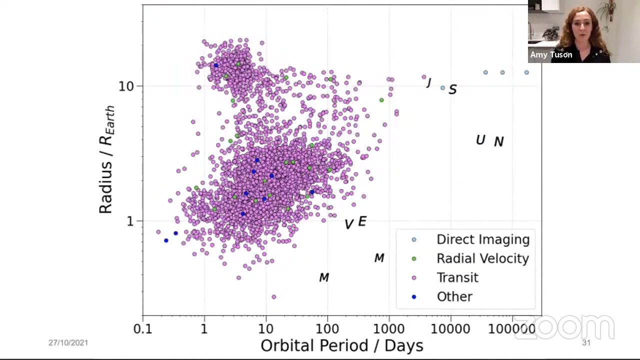 life. as we know it, At least three of the planets in the TRAPPIST-1 system are located in the habitable zone, and these could have the right conditions to support life. So let's go back to this period-radius diagram, because I want to point out one more thing that's important to note, The majority of confirmed exoplanets have much shorter orbital periods than the solar system planets. It's not that the planets in our solar system are particularly rare. It's just that our discovery methods are biased towards big planets orbiting very close to their host. 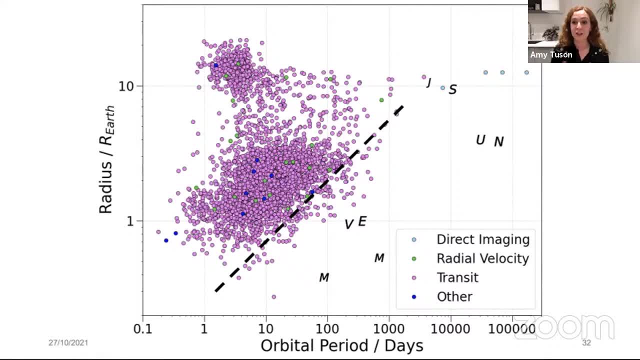 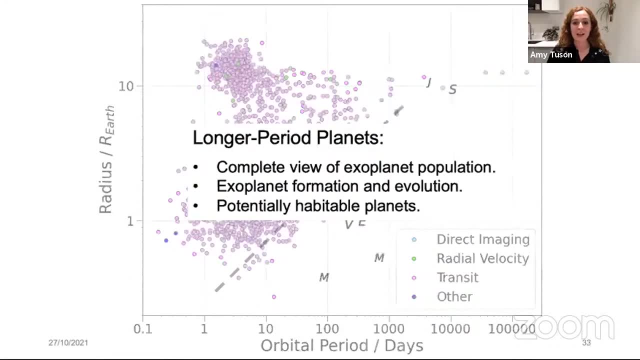 stars. They're not sensitive enough to find small planets on Earth-like orbits or large planets orbiting at Jupiter-like periods. So if we look at the solar system, we can see that the planets in our solar system have much shorter orbital periods. It's therefore really important we work. 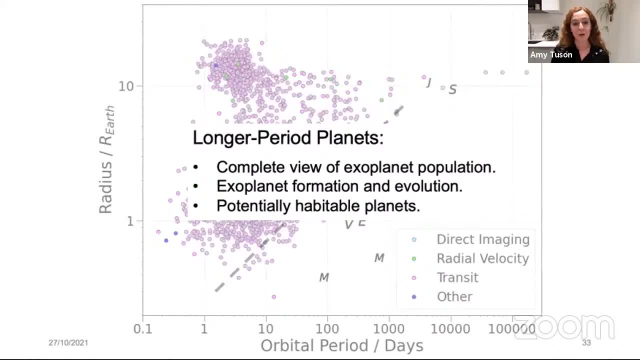 towards finding longer-period planets. Not only will this help give us a more complete view of the exoplanet population, but it will also help us to understand how exoplanets form, how they change over time, and it could reveal potentially habitable exoplanets. So that leads me nicely. 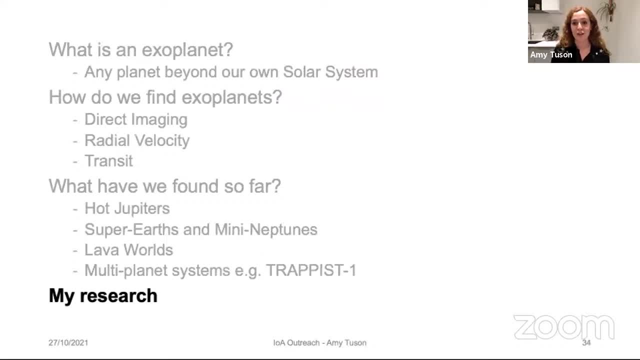 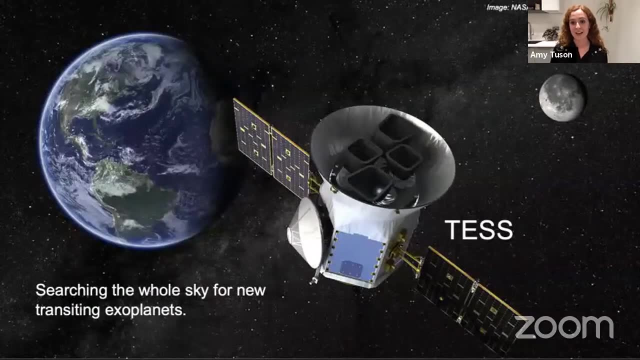 onto my research, So I work on the discovery of longer-period planets using a special space telescope called TESS. Now, TESS is a NASA satellite that searches for new exoplanets using the transit method. Between July 2018 and July 2020, TESS observed the whole sky and gave us 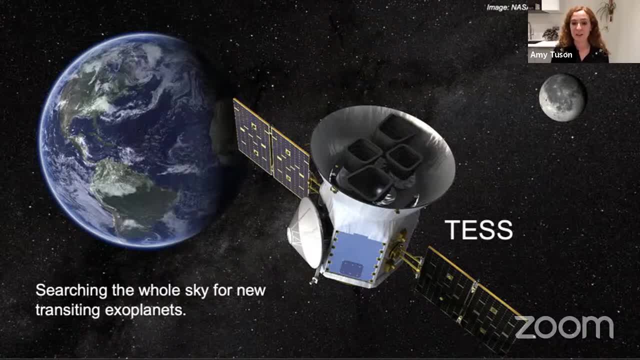 light curves for hundreds of thousands of stars. Most stars were only observed for 27 days, and this strongly favours the discovery of short-period planets. And that's because a short-period planet will show lots and lots of transits in a 27-day period. 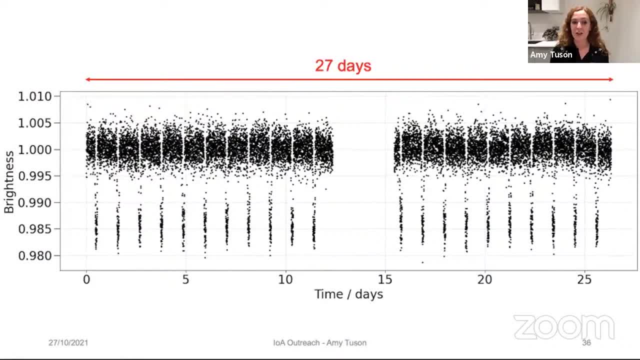 So here is a typical light curve from TESS. As I say, the whole light curve is about 27 days long, because this corresponds to the length of time for which TESS observed the star. There is also a planet in this data, So we see many transits because it is a short-period planet. 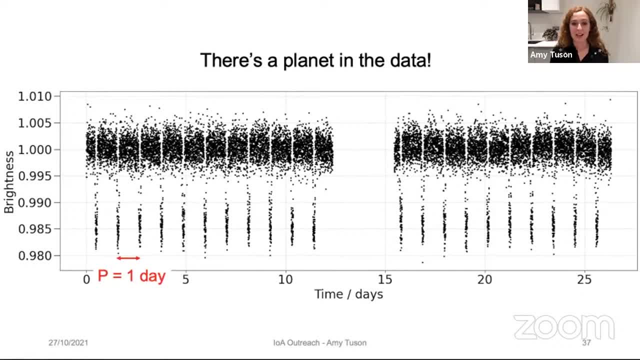 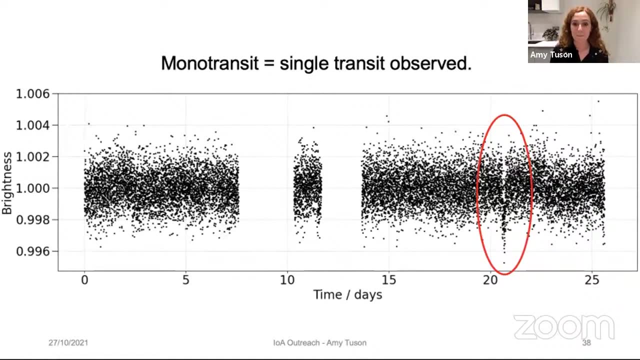 that orbits its star once per day. TESS is really good at finding planets like this, But what would happen if the orbital period was longer? If the period was longer, there might only be a single transit in the data, like this. This is what we call a monotransit. So what do we know about the orbital period in? 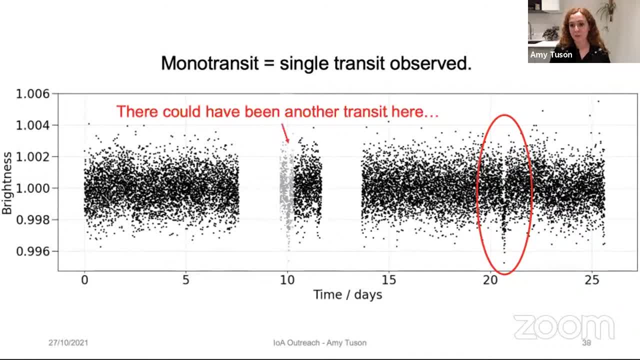 this case. Well, there could have been another transit here that was missed, Or there could have been another transit here, Or there might not be another transit for hundreds of days. My point is: all we can say for sure is that the orbital period must be longer than 10. 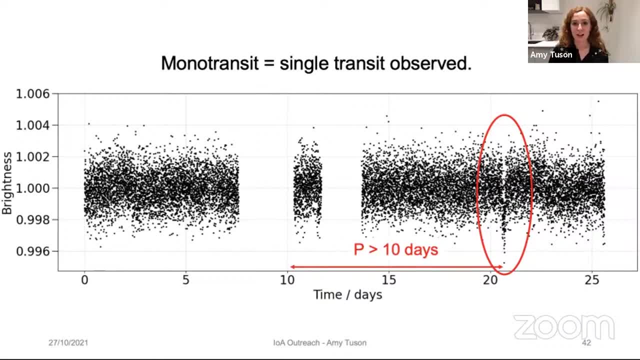 days. So monotransits offer a route to finding longer period planets, but we need more transit observations to find the orbital period and confirm that it is a real planet. So, luckily, TESS has been re-observing the entire sky since July 2020, and so we typically. 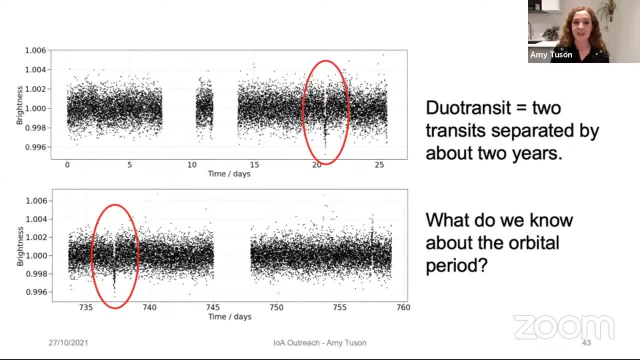 get another light curve for each star about two years after the first one. So the light curve with the monotransit that we've just looked at is shown at the top here and the new light curve is shown at the bottom, So you can see that a second transit of the planet was observed. 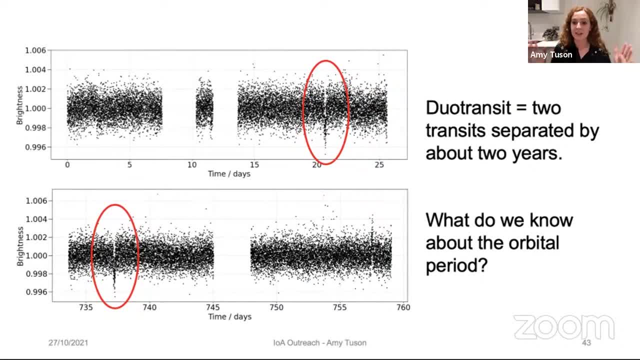 So what we now have is two transits of the same planet, Separated by about two years, and this is what we call a duotransit. These are the signals that I'm interested in, and they are the focus of my PhD research. 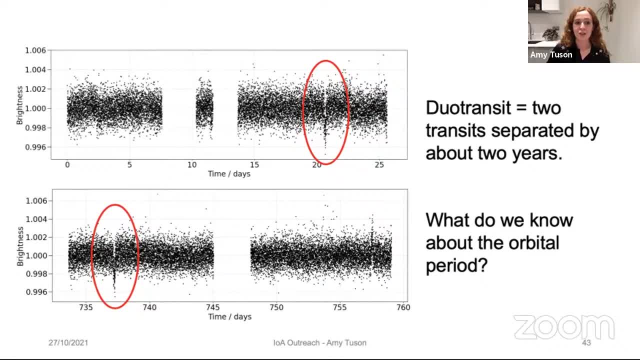 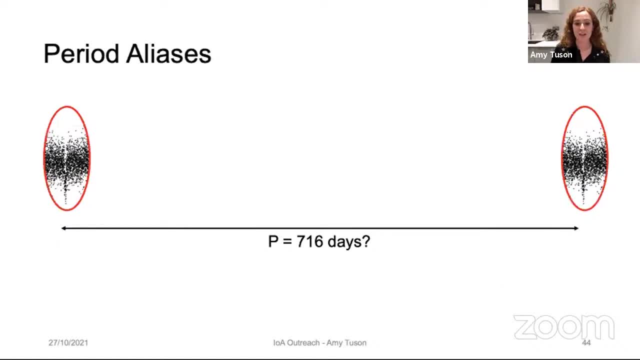 Duotransits are longer period planets, but the extra data helps constrain the orbital period. This is because we now have a set of period aliases, So the period of the planet could be the full separation of the planets, Separation between the two observed transits, which is 716 days. But if there was another transit that was not observed right in the middle, the period would be 358 days, And if there were two unobserved transits the period would be 239 days, And if there were three unobserved transits the period would be 179 days. 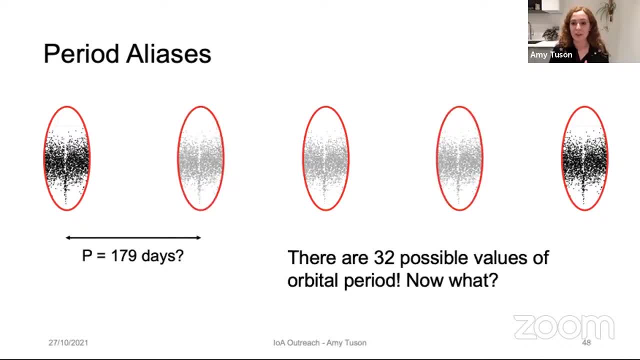 And we can keep going in this way. In total, there are three unobserved transits. There are 32 possible values of the orbital period. So remember when we had a monotransit, All we knew was that the period had to be longer than 10 days. 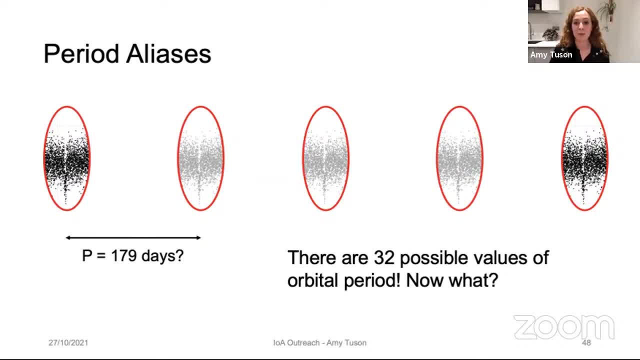 Now, with a duotransit, we know the period must be one of 32 values, So the second transit has helped us narrow down the period significantly. So what do we do next? We use another telescope to observe the star's orbit. 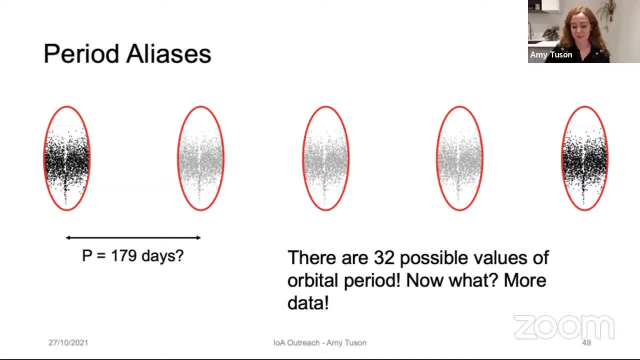 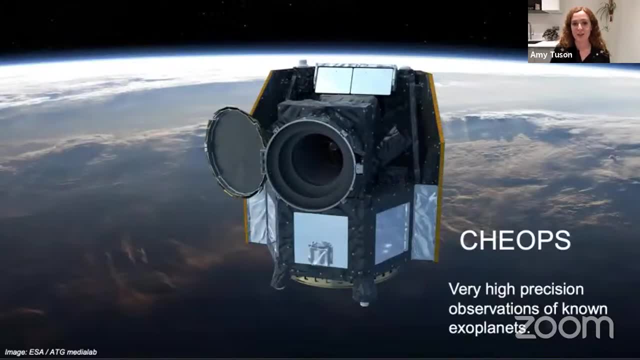 We use another telescope to observe the star's orbit. We use another telescope to observe the star's orbit. We start again and get even more data. To do this, I use KEOPS. So KEOPS is an ultra high precision space telescope that focuses on observing known 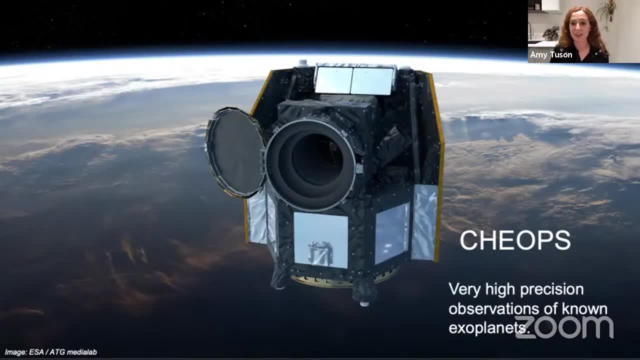 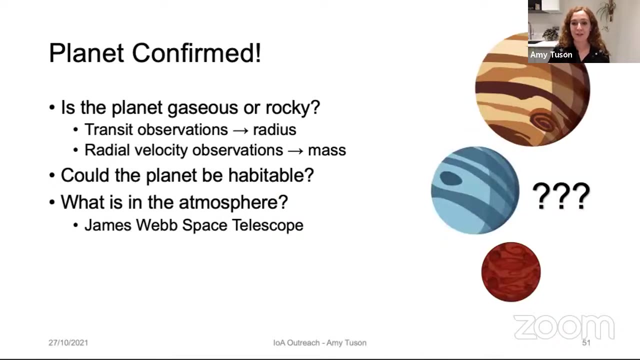 exoplanets rather than discovering new ones. With KEOPS, we can observe more transits of the duotransit and determine the correct orbital period. Once we know the orbital period, the planet is confirmed want to find out as much as possible about it, The first thing that we normally want to know. 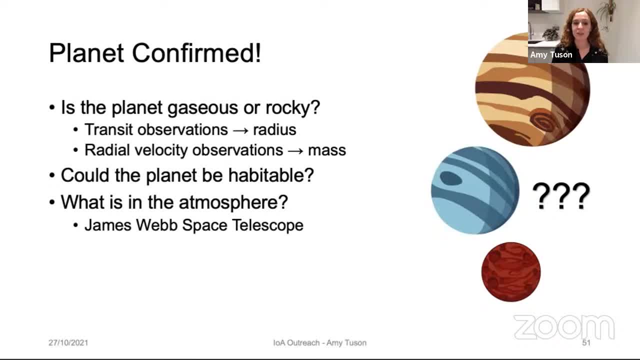 is whether the planet is gaseous or rocky. So from the transit observations we already know the planet's radius, but it also helps to get the planet's mass. Therefore, after a planet is confirmed by the transit method, we often go and observe it again with the radial velocity method. 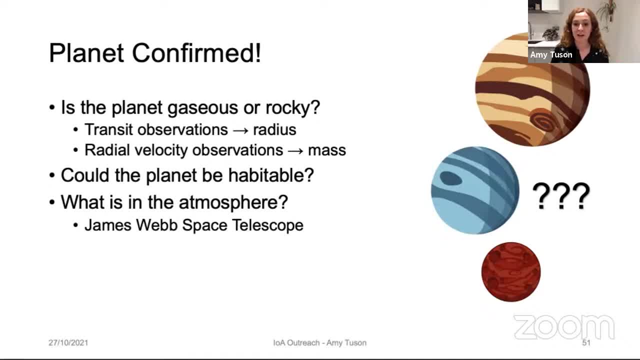 to measure the mass. With the mass and radius combined, we can then infer the composition of the planet. With the orbital period, we can also determine if the planet orbits in the star's habitable zone, and hence whether or not it could potentially sustain life. 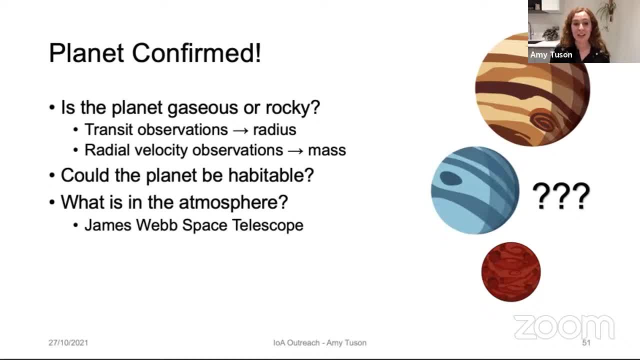 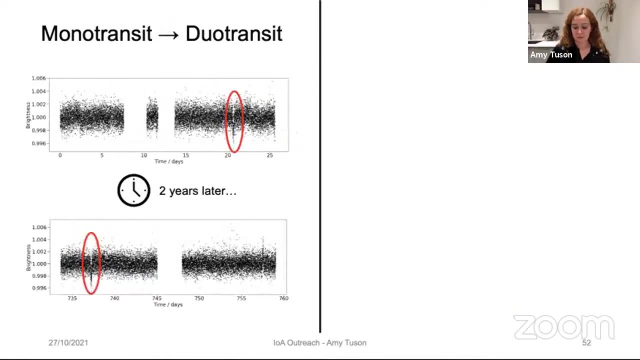 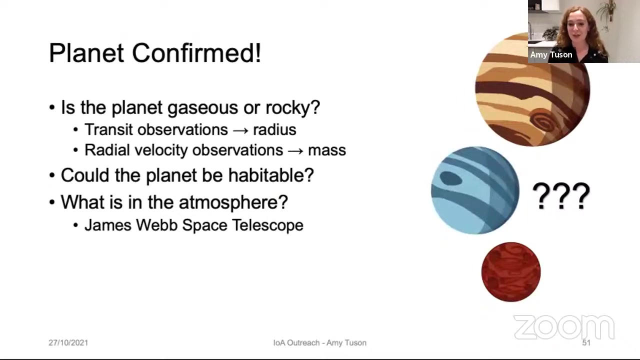 Finally, with more observations of the planet, we can even identify what is in its atmosphere and if there are clouds present on the planet. This is something that the soon to be launched James Webb Space Telescope will be able to do really, really well. Sorry, So I've explained how we can go from a test duotransit to a confirmed long period planet. 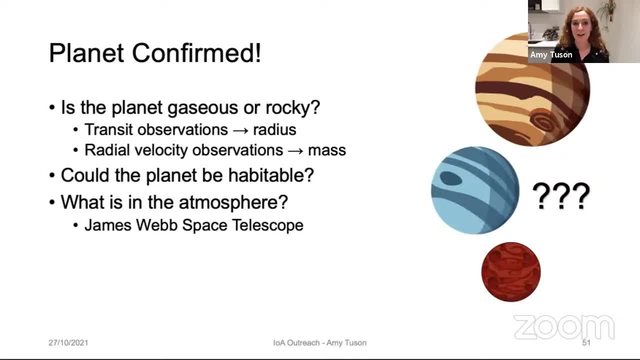 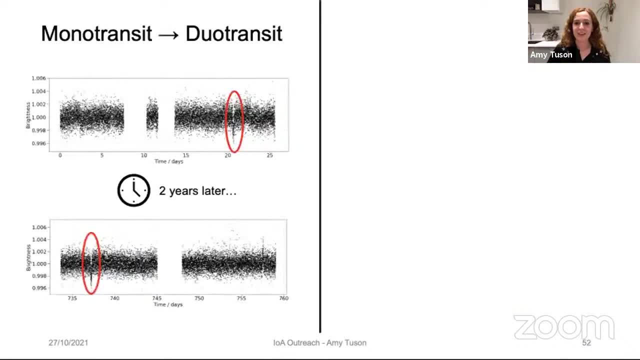 and that's almost the full story. but I've missed a key step out: How do we actually find the test duotransits in the first place? So most of the duotransits we found so far started off as monotransits and were then observed to transit a second time. 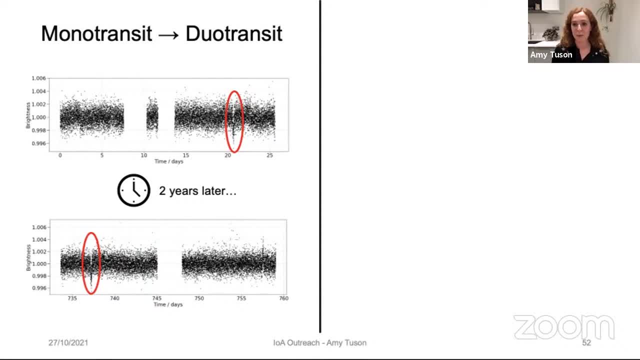 two years later, just like the one I showed you before. But there are more duotransits out there waiting to be discovered, and that's something that I'm working on. So, instead of waiting for a second transit of a known monotransit, I'm searching the test data for duotransits directly. 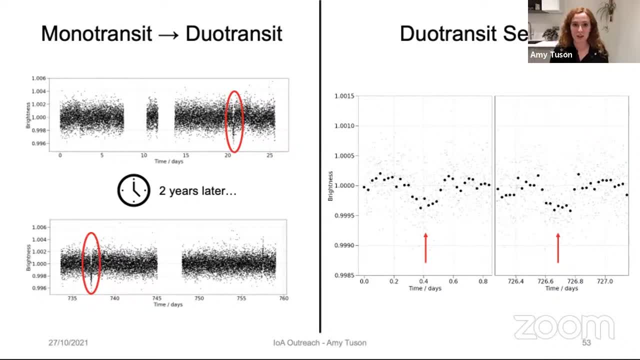 As I said, TESS observed hundreds of thousands of stars, so we cannot very easily search for duotransits by eye. Instead, we need to get a computer to do it for us. So I've created an automatic duotransit search that looks through thousands of TESS light curves for the 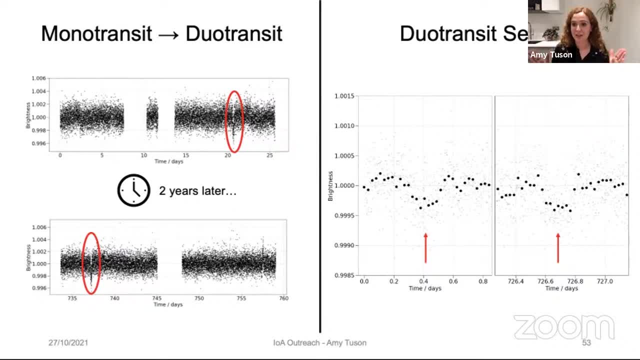 characteristic duotransit signal: two transits with a large gap between them. This search then returns a list of possible duotransits that I can then check. So on the right here I'm showing a duotransit that was discovered by my automatic search. 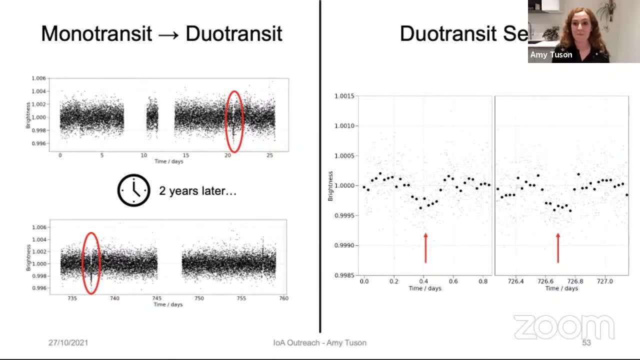 It's a shallow transit. so remember that means the planet must be quite small. And this is a particularly special detection for me, because a few weeks ago I confirmed that the planet was a small planet. I then confirmed it as a new exoplanet. So not only this, but it was the first exoplanet I've 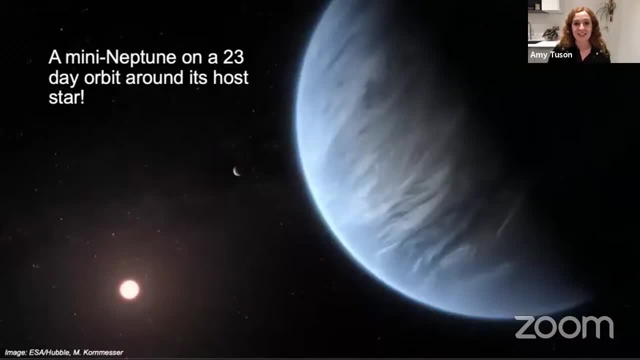 discovered, which was really, really exciting. It started out as a TESS duotransit with 38 possible values of the orbital period. Additional data then confirmed that the planet was a mini-Neptune with an orbital period of 23 days. 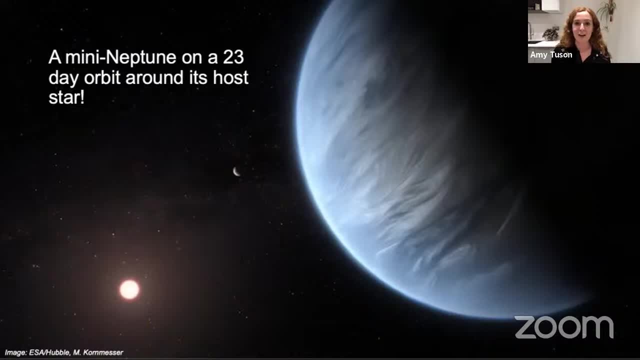 Now I told you at the start that my research was about finding longer period planets, and 23 days might not sound like a very long period, But remember, TESS only observes most stars for 27 days at a time, So a 23-day period is longer than it would normally be able to find. 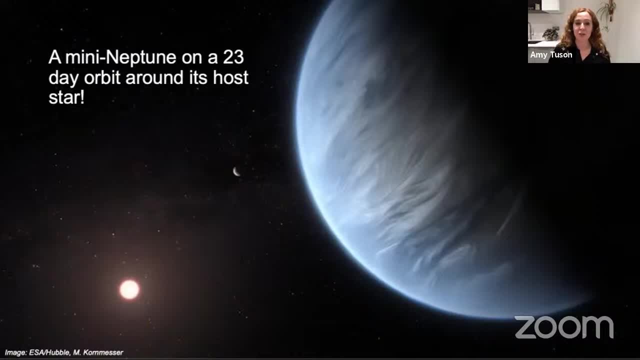 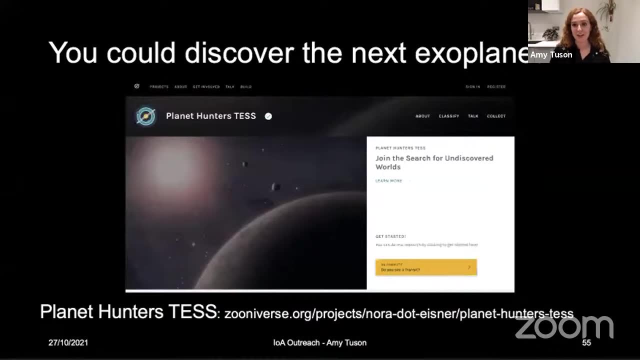 We're currently in the process of trying to understand as much as possible about this new planet, So I'd like to finish up by showing you how to join in the exoplanet search at home. So there is a project called Planet Hunters, TESS, which is a project that's been going on for a long time. 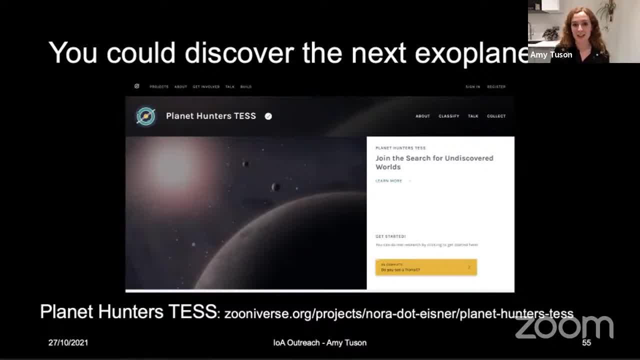 It asks the public to search TESS light curves for planets. As I've said, we normally have to use computers to search for transits because there's so much data, But the problem is computers can miss the more unusual transits that only a human eye can detect. So we therefore need your help If you join Planet Hunters TESS. 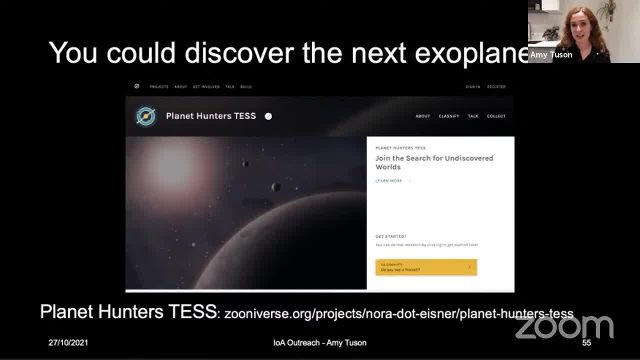 you'll be presented with light curves, just like the ones I've shown you today, and you'll be asked to scout the planet's transits, or any transits that you see in the data. You might just discover the next exoplanet. So I'm going to show you how it works with a couple of examples. 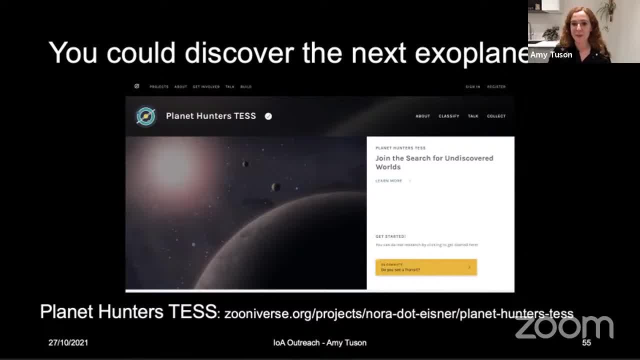 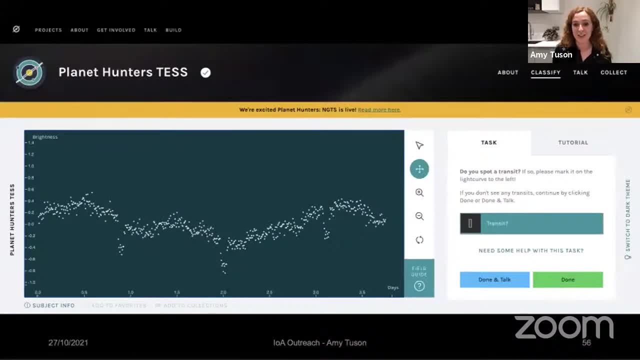 and I'm going to ask you to look for the transits and give you five seconds to see what you can find. So this is the first one, hopefully not too difficult. so I'll give you five seconds to find the transits. Five, four, three, two, one. 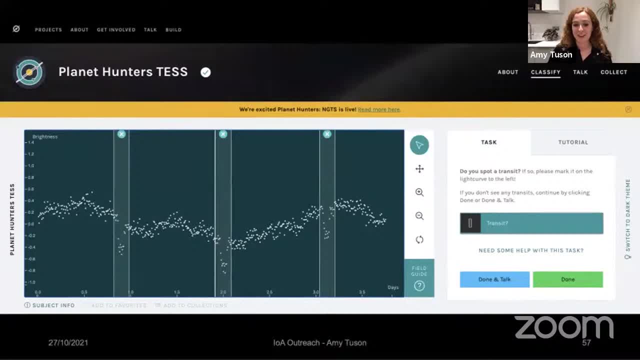 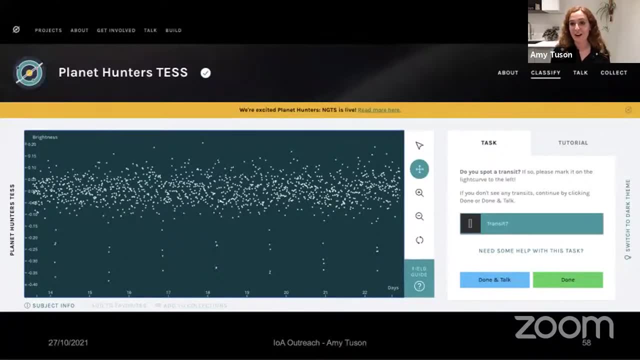 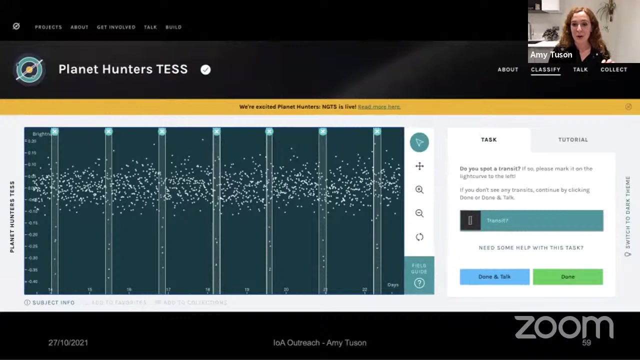 are. There are three transits in this light curve. Okay, another example. So how many transits can you see in this light curve? Another five seconds, Five, four, three, two, one. So if you counted seven transits, then you're correct. Okay, so one slightly more difficult example to end on. 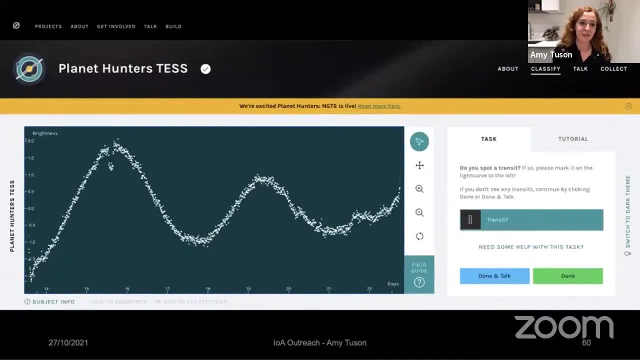 What can you see in this light curve And why does it look different to the others that I've shown you? And are there any transits? So I'll give you another five seconds. Five, four, three, two, one. So there is one transit in this light curve. The other variability that we see here: 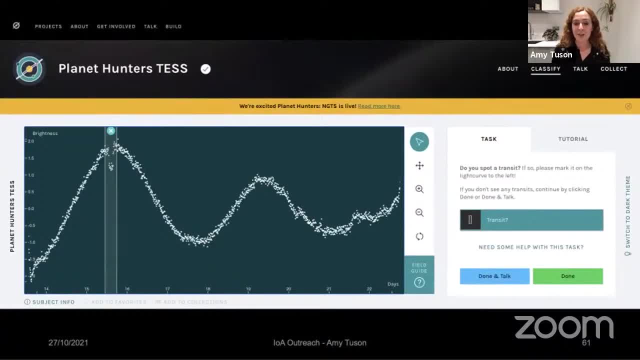 is coming from the star itself, And that's because stars can become periodic, brighter and dimmer over time. So when you have a light curve like this, that's something that you need to look out for, And you need to be able to learn the difference between the stellar. 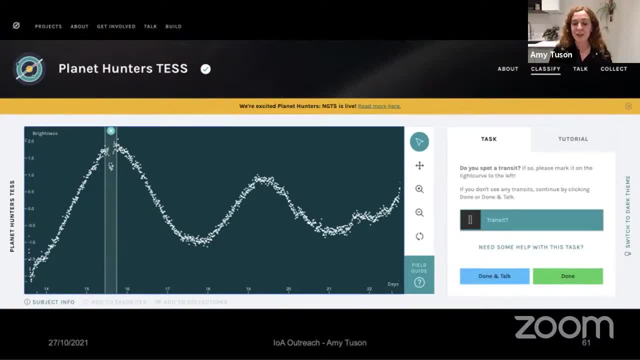 variability and the transits. So if you've enjoyed searching for these transits, or you know somebody else who would, then I really recommend that you get involved with Planet Hunters. So with that I'll leave a summary of what I've spoken about here. Thank you so much for listening, And I'm 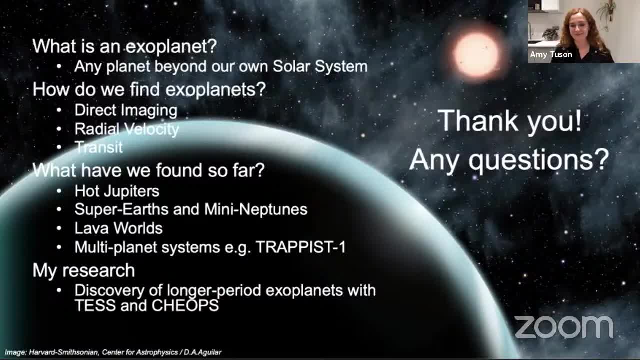 happy to take any questions that you might have. Wonderful Amy, Thank you so much. It was really fun at the end spotting the transits. I can see people- some people in the YouTube chat were joining in- Yeah, So yes, if you have any questions for our speaker, please pop them down here in the YouTube chat. 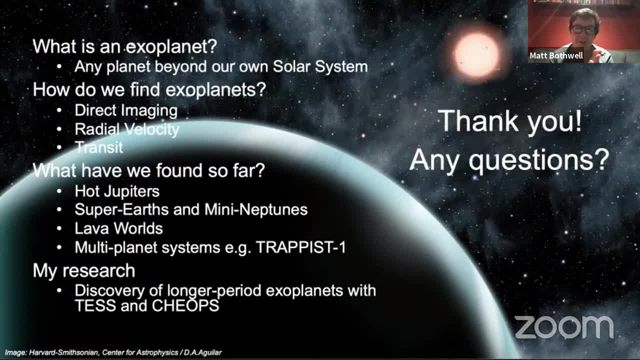 And I will make sure she sees them While people are typing their questions. I've got a question to start with, actually. So you showed that light curve data where you said you can't really see a transit in there, but you promised they were there. How do you know? 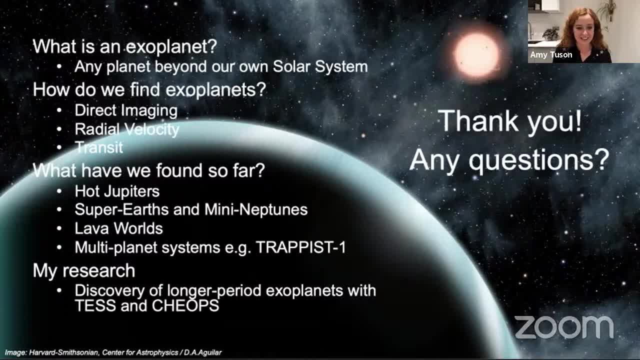 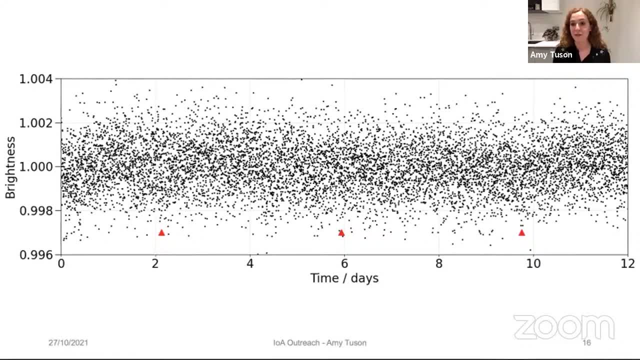 Ah, so I will go back to that light curve. So it's this one. So the reason: we know there's transits there. this star has been observed for hundreds of days continuously, So I'm only showing a really small section of it here, And in this really small section we have three transits. But you can see 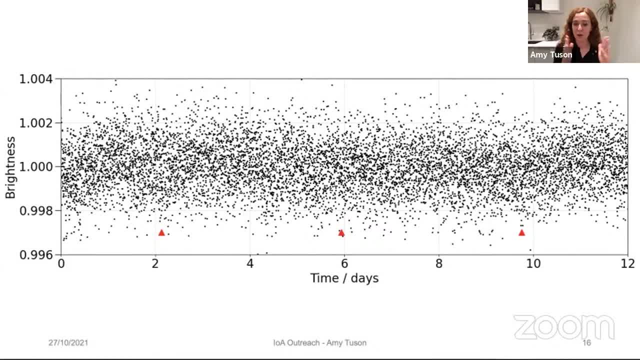 that the period of this planet is about four days because they're quite close together. So in our hundreds of days of data we have a lot of transits, So we can see that the period of this planet is transits. So imagine, every four days, for hundreds of days, we have a transit. So what we can do is by 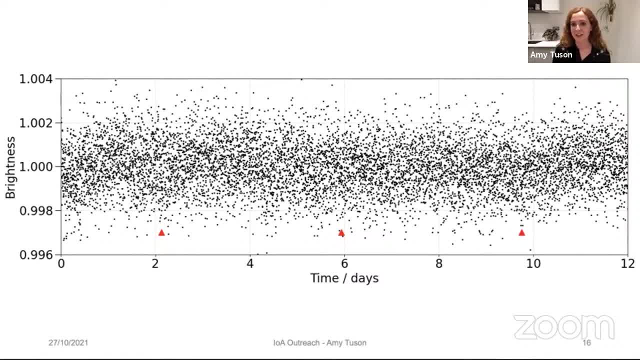 stacking them on top of one another, the transit begins to reveal itself. So with only three transits you can't really see it. But if we combine lots and lots of those transits, that's how we can find them Wonderful. That makes sense. And you mentioned JWST. I assume everyone in the exoplanet community. 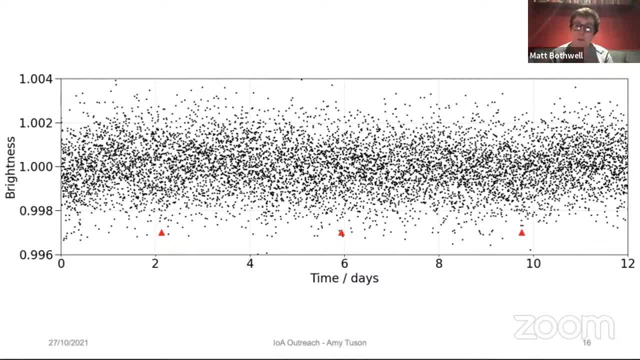 is looking forward to JWST. Can you maybe just tell us a little bit about what this new telescope is going to be able to do for us? Yeah, I think it's going to be a lot of fun. It's going to be a lot of fun. It's going to be a lot of. 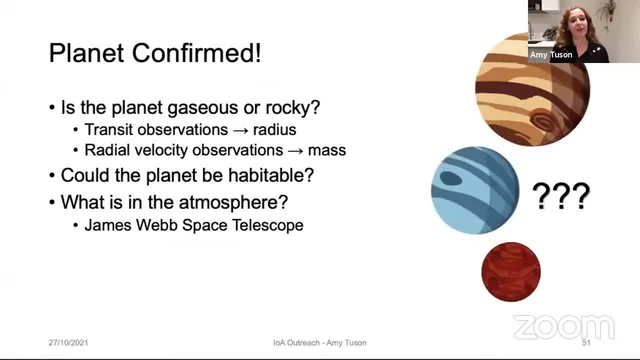 fun. So JWST is something that I've mentioned here- that once we know a planet exists, so JWST won't be able to discover new exoplanets for us. What it will be able to do is tell us more information about the exoplanets that we know. So when we found a planet, as I say, we want to, 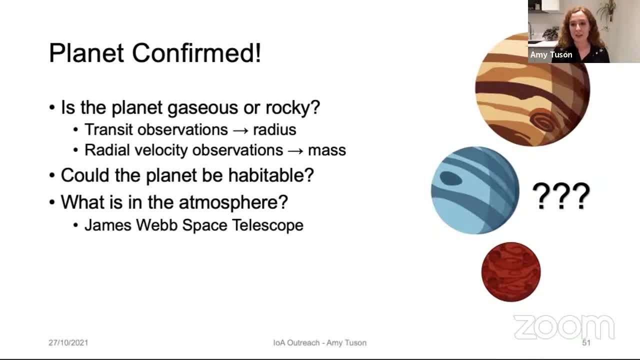 find out as much as possible about it And JWST will be able to observe the atmospheres of those planets. So it will be able to look at the planets that we found. And if you imagine that these planets have a lot of gas around them, especially the gas giants, they're mostly gas, So JWST can. 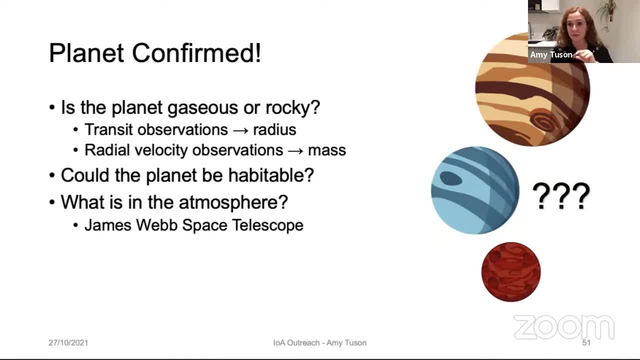 peer through that atmosphere and pick out certain molecules. So, for example, we have detections of water vapor on other exoplanets and we have detections of methane and things like that. And it becomes really interesting because some of these molecules can be biomarkers, So that 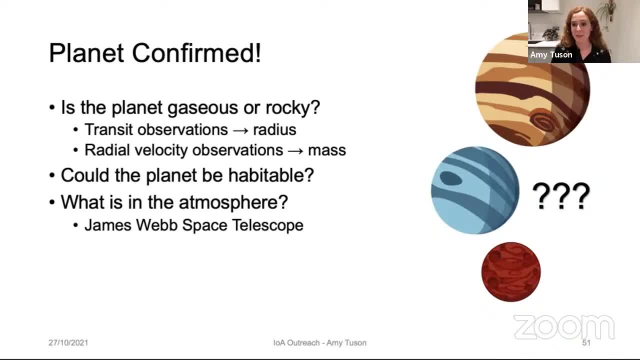 means that there are certain things that we can look for in the atmosphere of a planet that could perhaps suggest the evidence for life on that planet. So obviously it's very, very hard to prove definitively that there is life there, But there are certain clues that can tell us that. 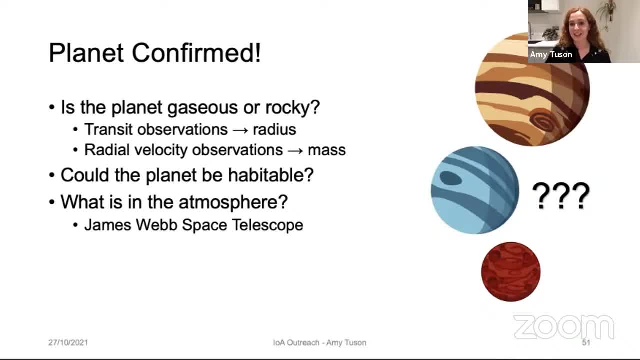 perhaps there could be something there. So JWST is really exciting like that, And it will be the first telescope that's going to be this sensitive, So it's going to be able to give us lots of interesting data that will tell us about their atmospheres. 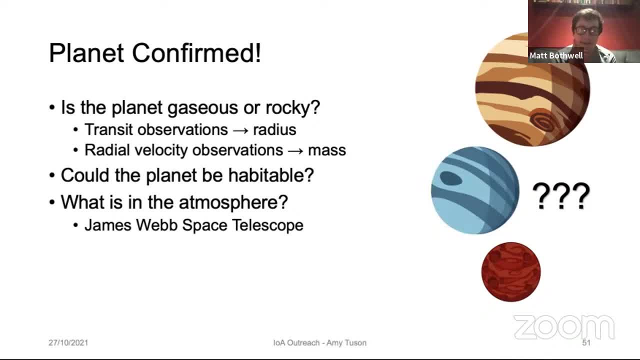 Amazing, Thank you. Lots of people in the chat saying thank you for the fascinating talk. Kieran wants to know why would a star vary in brightness? Ah, so actually this might be a good picture to show for that. So do you remember I showed this? 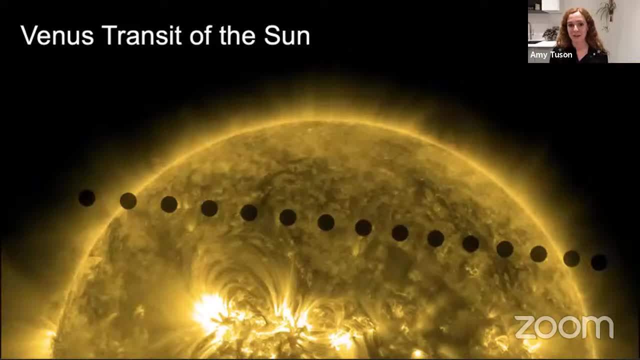 picture, And this is our own sun, with Venus passing in front of it. So do you see all of these features on the sun's surface? So we have some bright regions and we have some darker regions. So what happens is stars rotate. 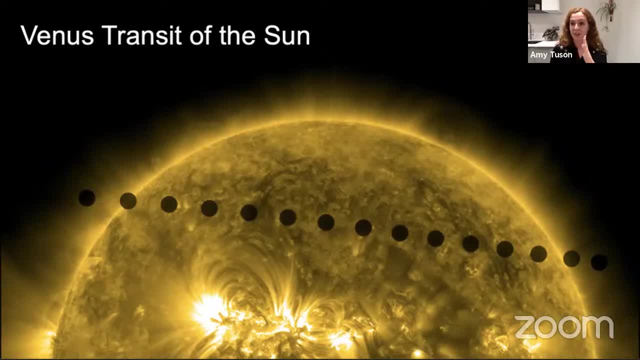 So the star itself is rotating and showing us different sides. So if you have one of these bright areas and one of these dim areas and the stars rotating, we then track the brightness of that star over time in our light curve And what we see is, as the bright regions come in, the 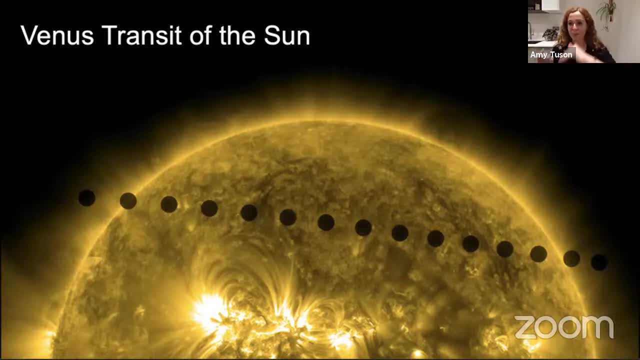 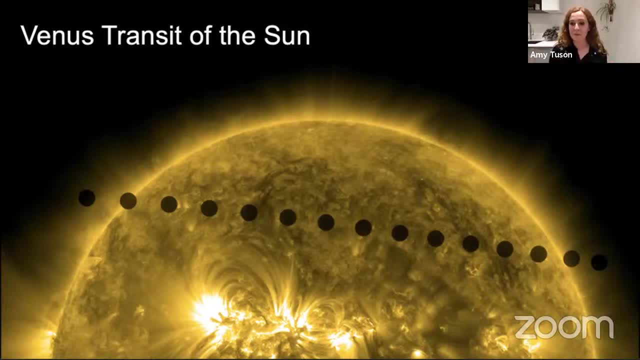 very wiggly And then some of them rotate really slowly So we'll get much more kind of flat light curves, And some of them don't really have much activity at all. So like some of the other ones I've shown that were quite flat, So some of them don't really have this effect. So every star is: 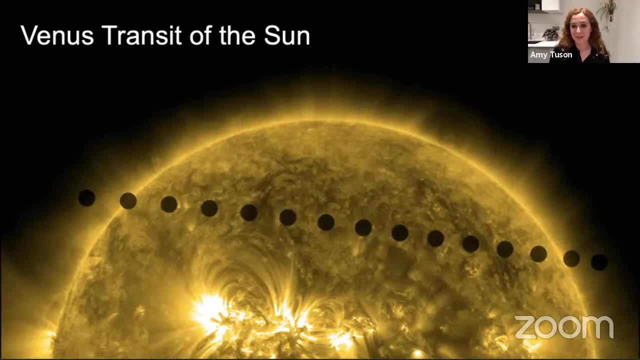 different. in that respect, Wonderful, Thank you. A question from Nick. Nick has noticed that when you hear the data about the different types and characteristics of exoplanets, very few of them are close to the Earth's values. Can you explain what's going on there? Yes, Yeah, So I assume. 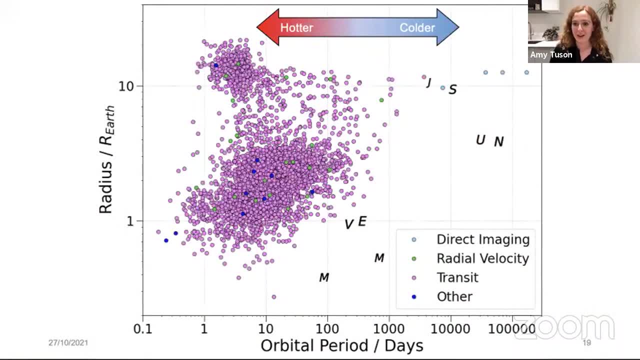 we're looking at this plot here when we talk about that. So, yeah, you're right, So the Earth is down here And obviously there's not really any exoplanets that we found. There's a couple that are close but still not at the same position, And that's because of something I mentioned. 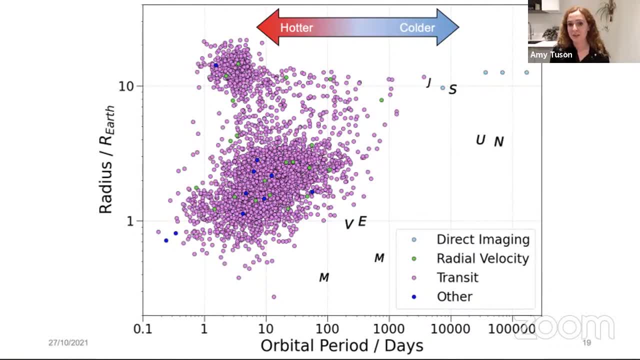 that our detection methods are really biased towards big planets orbiting close to the star. So we're good at finding hot Jupiters. So this cluster of hot Jupiters up here it makes it look like there's a lot of them, doesn't it? But actually we think hot Jupiters. are quite rare. We don't think that they're very common. It's just that we're really good at finding them because they're short period and big, And once we get down here we have short period and small. So we're still OK at finding them because there's so many transit features in the data. 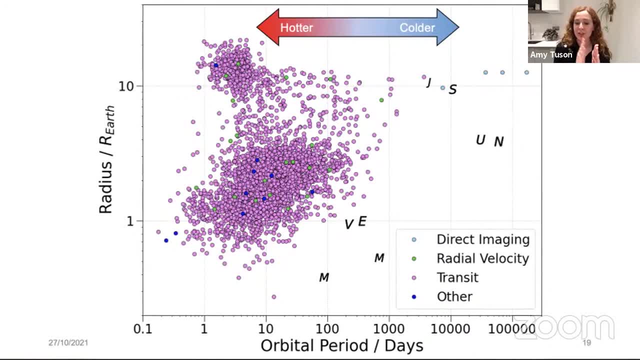 So remember how I said that? Yeah, So we're good at finding them because they're short period and small. And once we're down here, we're still OK at finding them because they're short period and small. So our experiment was done in a way in which we had no need for وس. 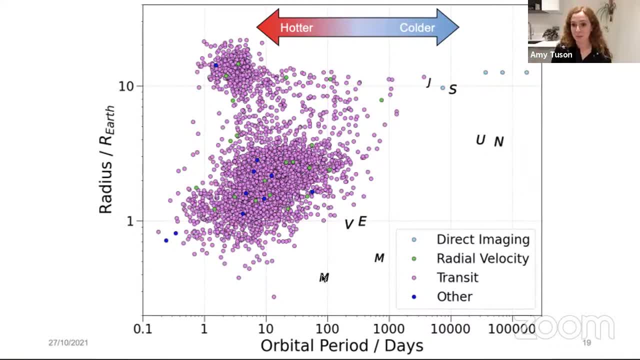 w亘 gap between our exoplanets And what I said. when we have small planets, what we do is we want to stack lots and lots of transits on top of one another so that we can find them. But when we have a long period small planet, we might only have two or three transits And with 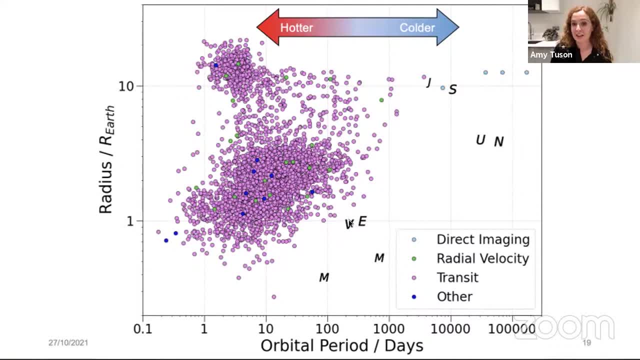 only two or three transits of a small planet. we simply aren't able to find them. So we really need to figure out a way to be able to find more exoplanets over here And the research I'm doing, the planets i find are more, you know, like this region here potentially, but getting out here. 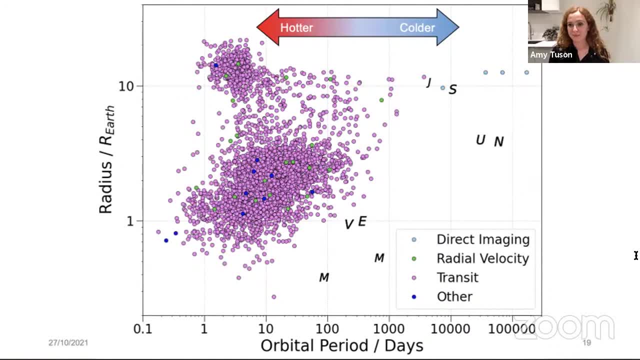 is going to be much more difficult. um, wonderful, thank you. uh. one last question, um, and that's something else comes through that last question, um, from stefania. um, who thinking about those kind of citizen science, uh, data sets you were talking about before. are any of these data? 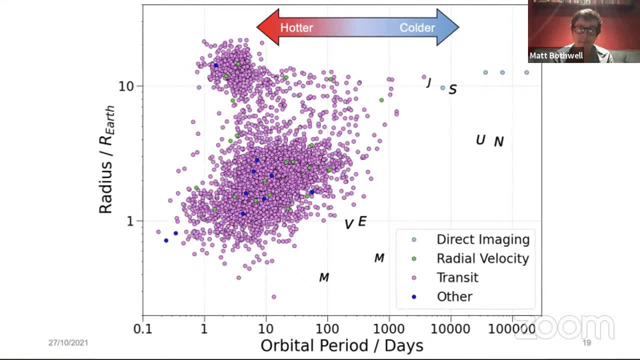 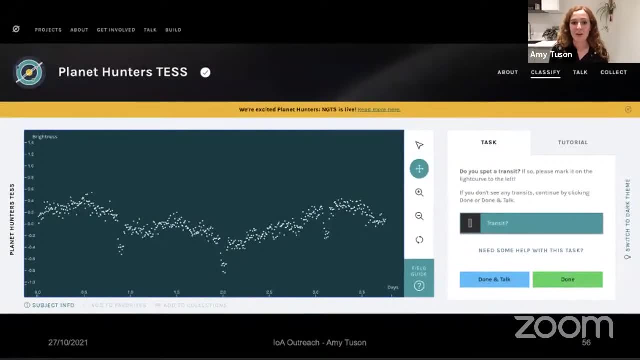 available for people to download and have a play with themselves. yeah, absolutely so. this is planet hunter's test, as i say. so, if you google this, you'll find this web page, and planet hunter's test shows you this kind of interface where you will be shown a light curve, just like this, this. 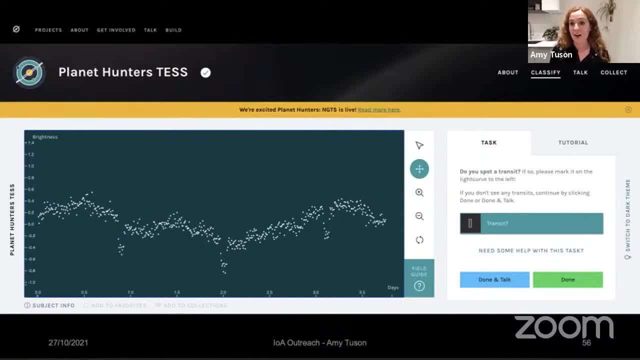 is a screenshot of the web page and you'll then be asked to highlight the transits, so you simply click on the image and drag over them. but if you want access to the data itself, um, the test data is all intact, um, so if you give a google for tests, um, it's run by mit, um in the states, and you should be able to. 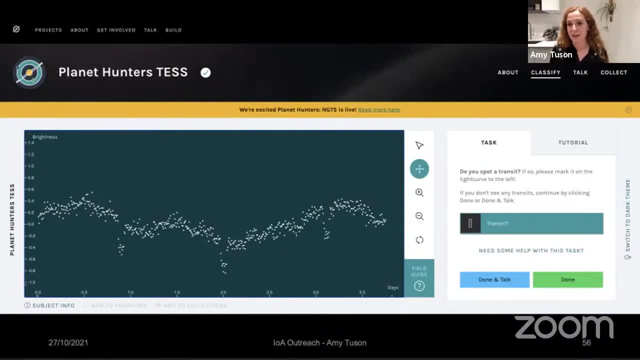 find um the public data. all of these light curves are available, so if you want to, you can go and search for planets yourself in absolutely any of them. wonderful, thank you so much. i i suspect there'll be some people going and doing this um after your talk, many people saying how much they.